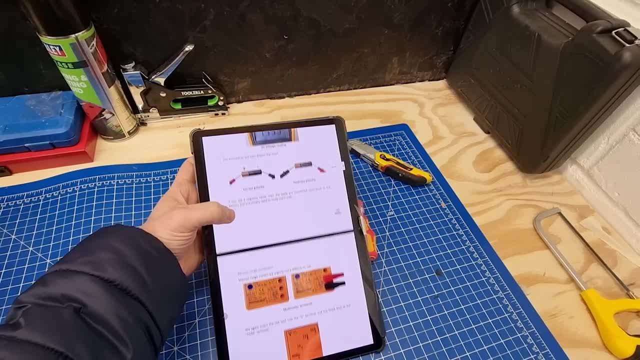 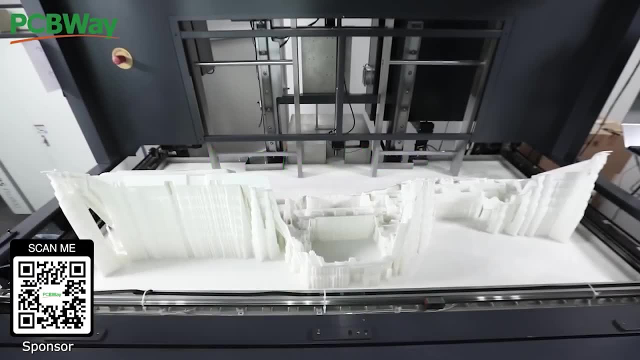 You can even download my Multimeter PDF Book 2 and support the channel Links down below for that, along with links to our sponsor, PCBWay, who offer everything from circuit boards, 3D printing, CNC machining, injection, molding and even sheet metal. 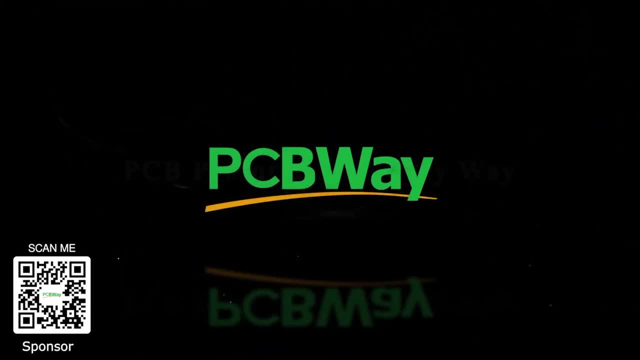 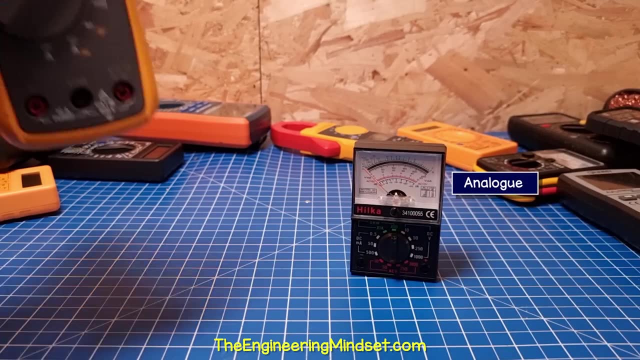 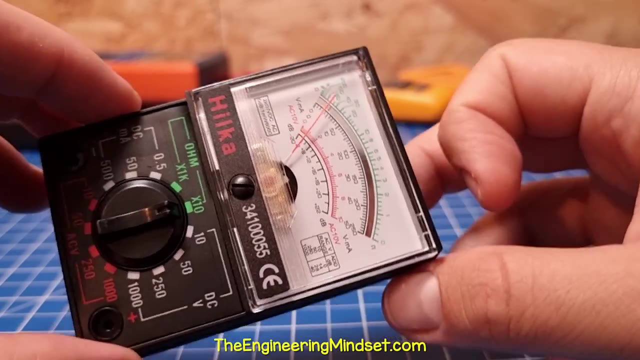 fabrication. Do check them out. links down below. There are a lot of different multimeter designs, but basically we just have the analog and the digital versions. Analog multimeters use a dial which is horrible to use and difficult to read, and they usually just have a few basic functions. 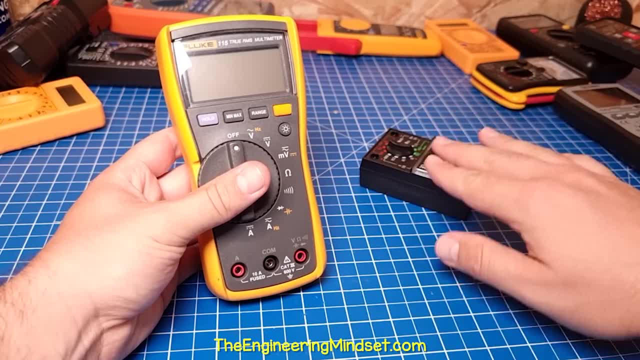 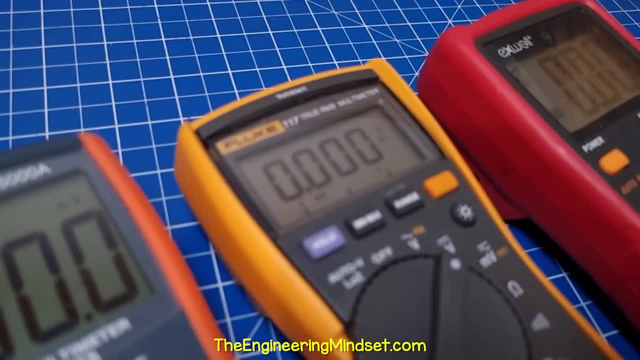 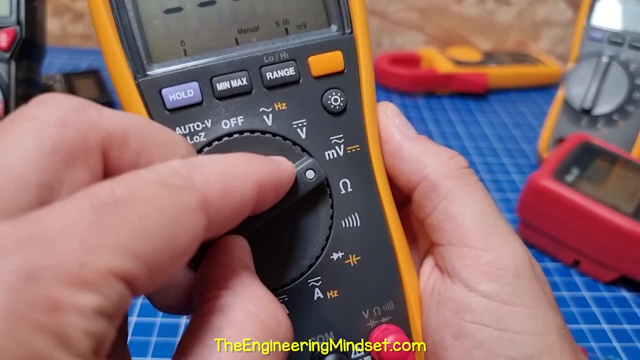 Hardly anyone uses these anymore. I can't stand them and I'm not going to cover them in this video. Instead, we're going to use digital multimeters which have digital displays. These are precise, very easy to use and usually have a lot more functions. 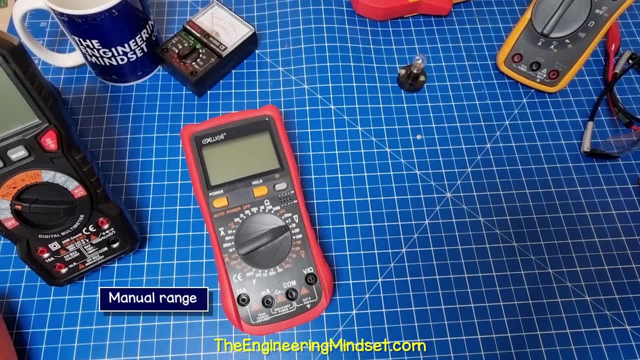 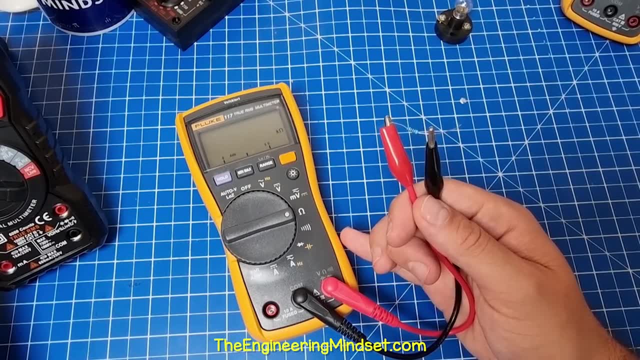 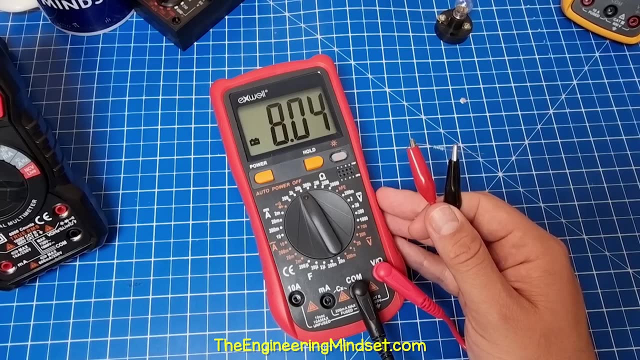 We have two main types of digital multimeter. There's the manual range and the auto range. With auto range we just select the function and the multimeter will tell us the answer. But with the manual range version we have to select the correct range to get the correct answer. 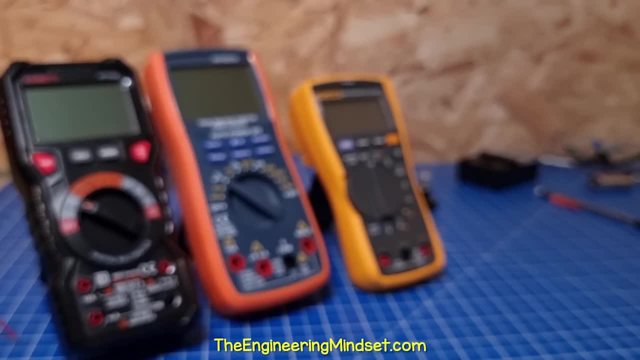 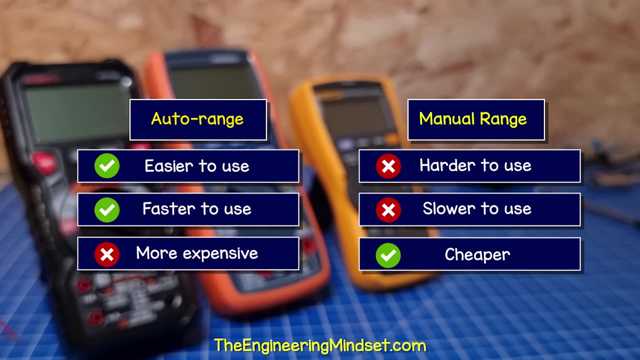 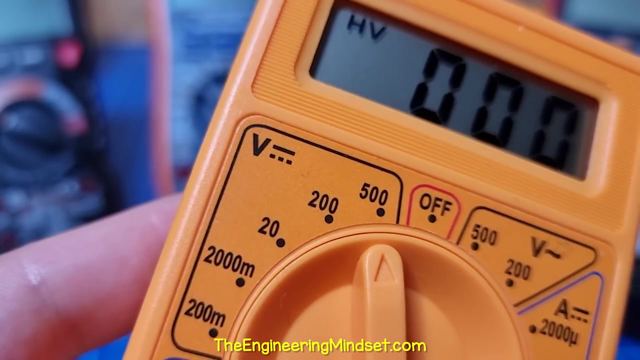 We will see how that works a little later in the video, But auto range are the easiest and the fastest to use. However, they are typically more expensive. I'll leave my multimeter recommendations in the video description for you. However, all multimeters have the same basic functions of reading voltage, current and 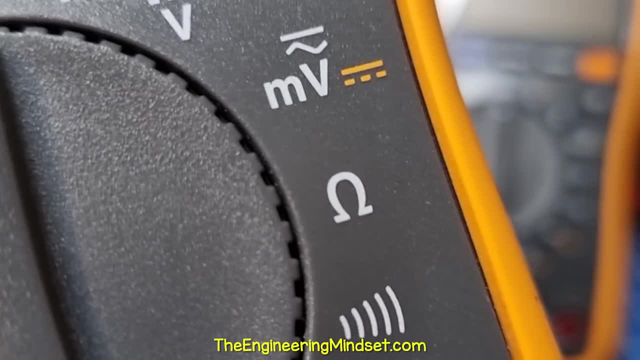 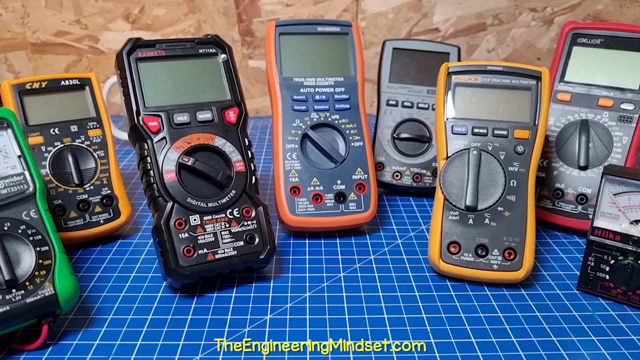 resistance. However, they all have the same basic functions of reading voltage, current and resistance difference. Different multimeters will have more advanced functions for things such as capacitors, transistors, diodes, temperature, etc. We will cover all of these, but let's get started with. 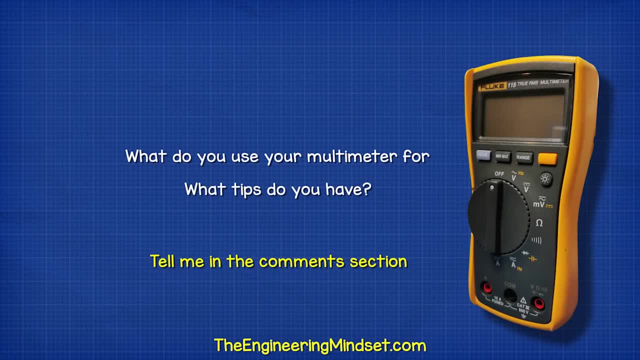 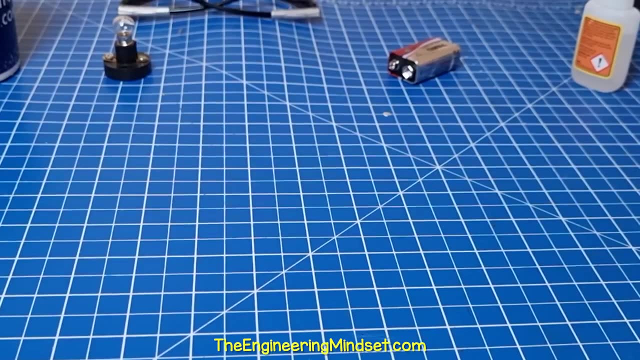 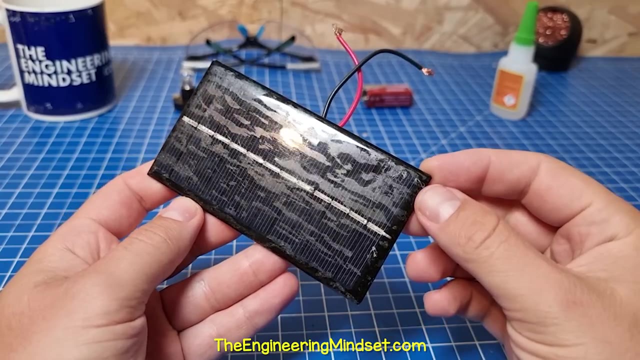 DC voltage. What do you use your multimeter for or what tips do you have? Let me know. in the comment section down below, DC voltage is represented by this symbol. We find this type of electricity with batteries, solar panels and almost all of our electronic devices With DC. 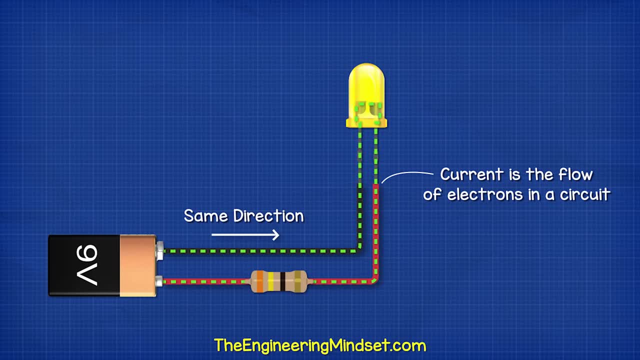 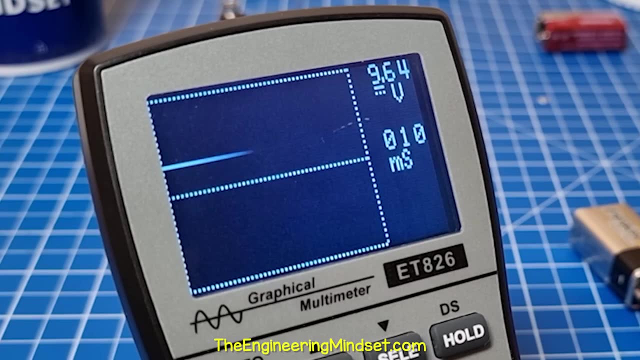 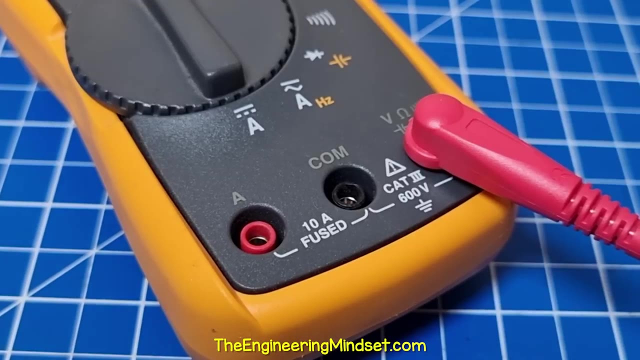 or direct current electrons flow in one direction. Think of it like the flow of water in a river. That's why our oscilloscope shows a straight line when we connect it to a battery and that's why we use this symbol. We place the red lead into the V terminal and the black lead into the COM. 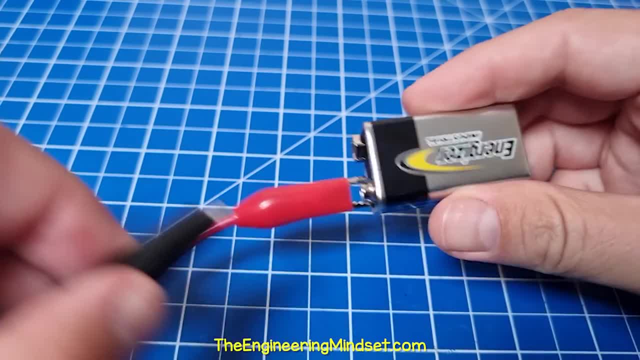 terminal. Then we connect the red probe to the positive and the black probe to the negative. We connect the red probe to the positive and the black probe to the positive. Then we connect the red probe to the negative terminal of the battery On the auto range. 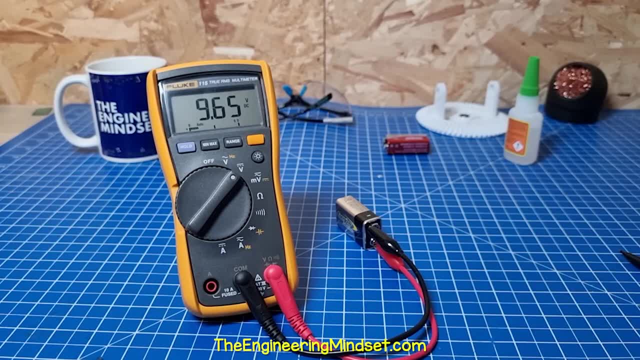 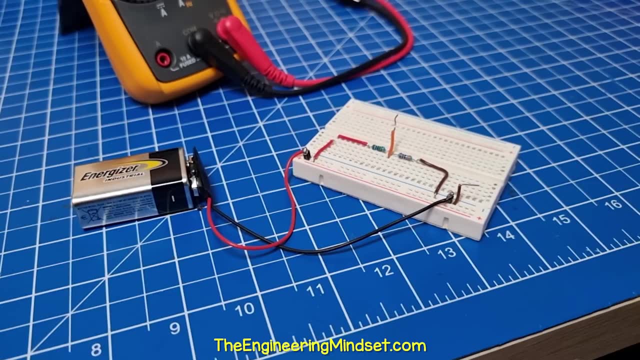 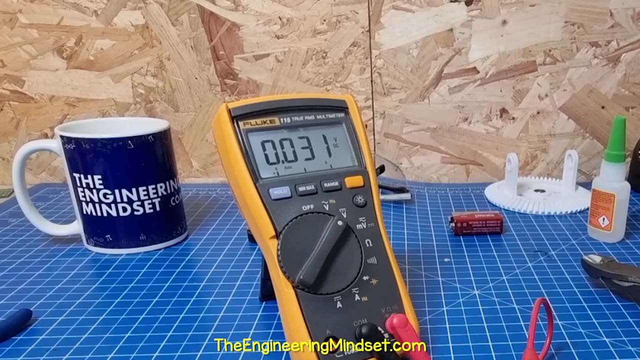 multimeter. we just select the DC voltage setting and it will instantly tell us the answer. If you see a negative number, you just need to swap the leads over. Here I'm testing a simple voltage divider circuit. We can see a reading of 0.031 volts, which is 31 millivolts We can switch to. 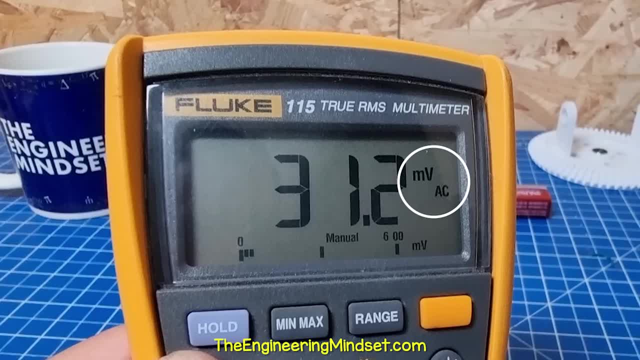 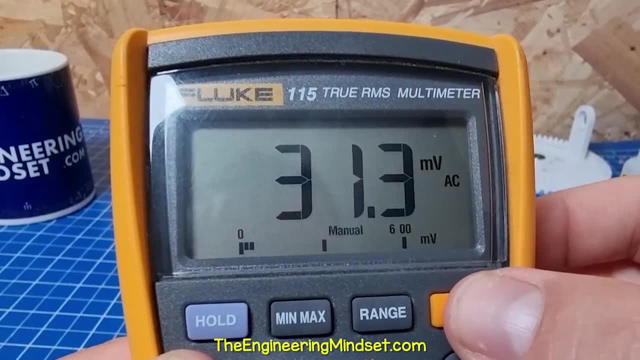 the millivolt setting for more precision. This particular device defaults to a higher voltage than the AC millivolts and it indicates that we need to press the yellow button to switch to DC millivolts. With the manual range version, we have to select the correct scale. That's quite easy. 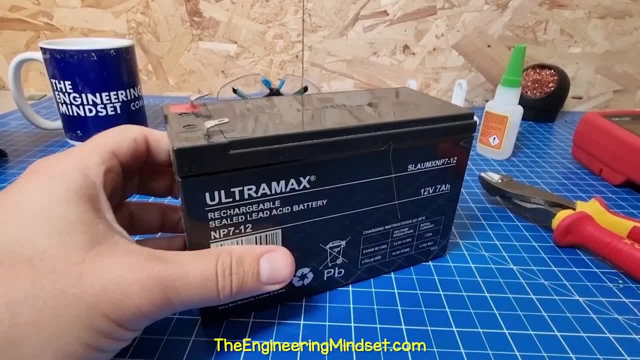 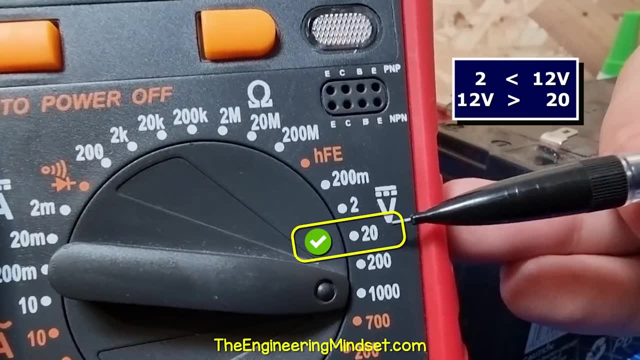 We just select the next number up. For example, this battery is rated 12 volts, That's higher than the 2, but less than 20. And so we use the 20 scale. This battery is rated 1.5 volts, That's. 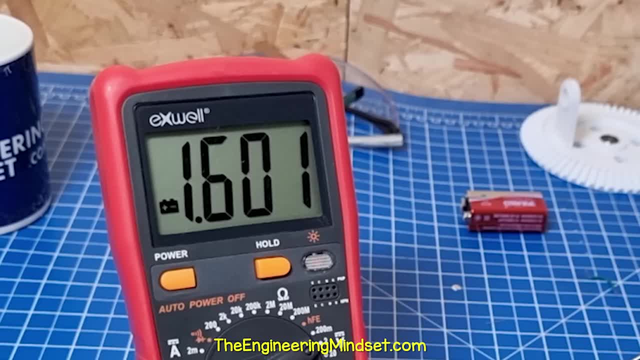 less than 2, so we use the 20 scale. This battery is rated 1.5 volts. That's less than 2, so we use the 2 scale. But what if we don't know the voltage? How do we choose the correct scale? 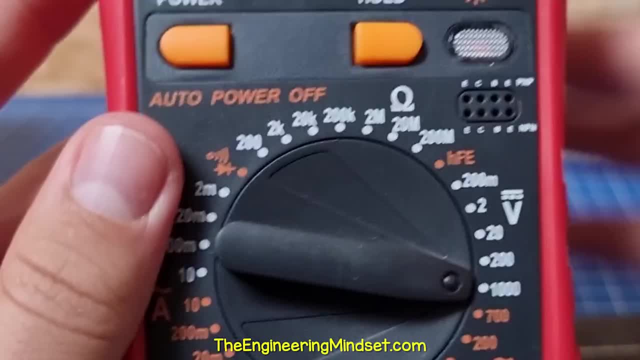 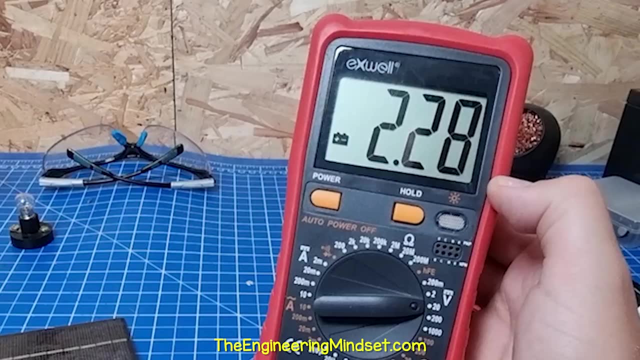 Well, that's easy. We just start from the highest value and turn the dial until it changes to a 1. That means we have gone too far, So we turn it back to the next position and that will give us the answer. We can also measure voltages in a circuit. 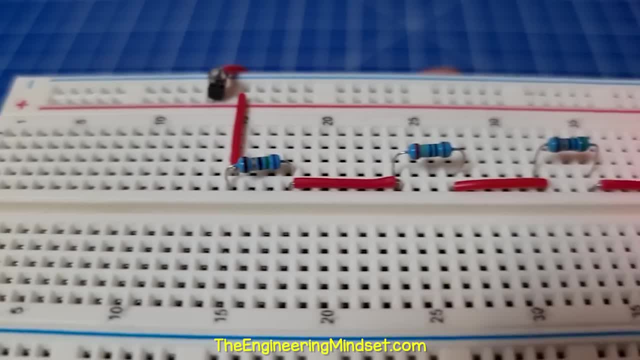 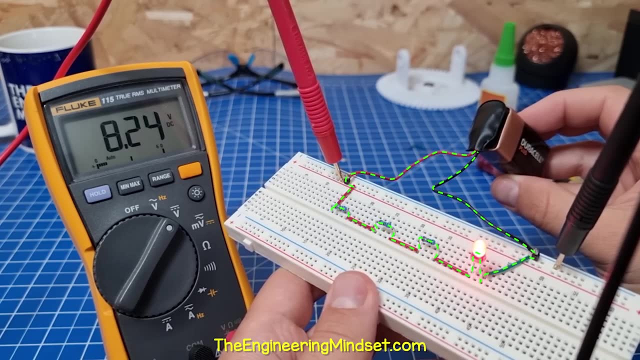 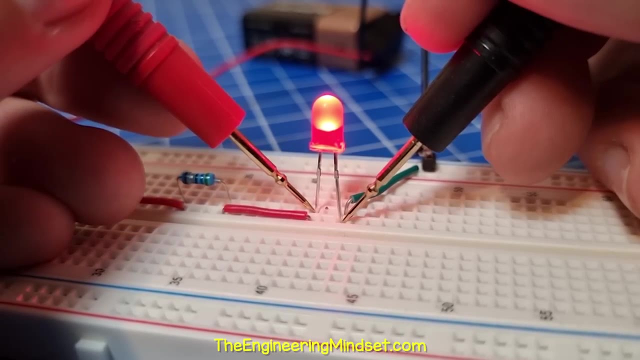 For example. here I have a basic prototype board with some resistors and an LED. I can read the voltage of the circuit by measuring across the positive and the negative. I can also check the voltage at any point in the circuit by connecting across individual components. We can check the. 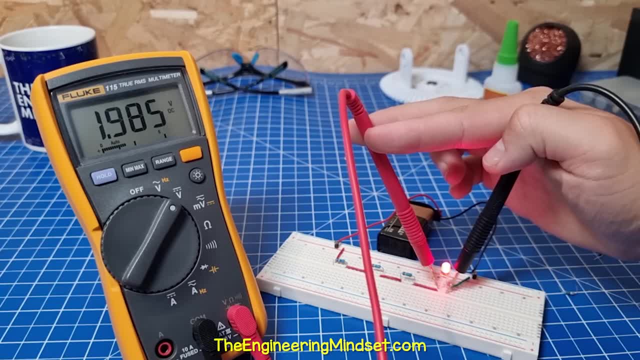 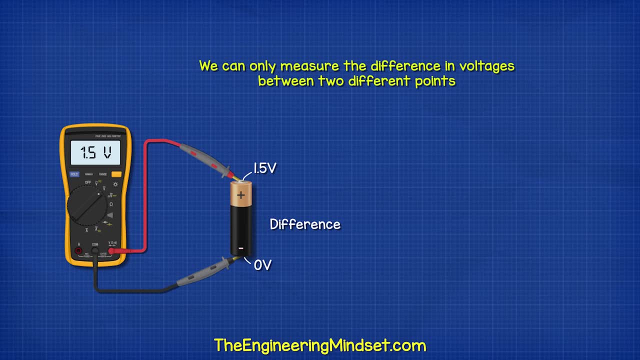 voltage drop of that component, although it must be powered in order to do this. Remember, we can only measure the difference in voltages between two different points. If we try to measure the same point, we won't read any voltage because there is no difference. 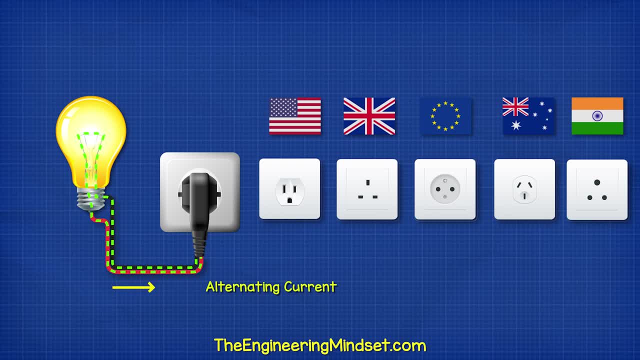 The electrical sockets in our homes provide AC or alternating current. This is different than DC electricity, which we get from a battery. With AC, the current alternates direction, flowing forwards and backwards. Think of it like the tide of the sea. 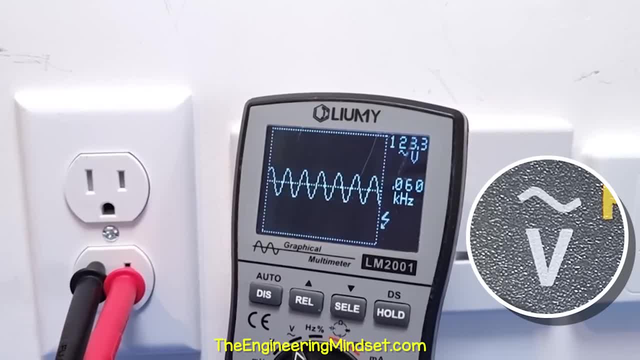 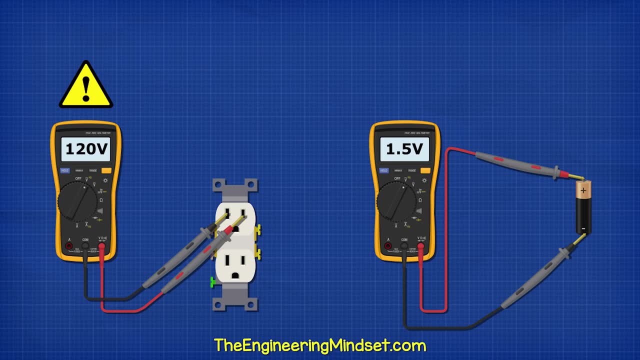 So our oscilloscope will show a sine wave for AC, which is why we use this symbol. This is a much higher voltage than a battery. If you have a battery, you should be able to measure the voltage at any point in the circuit. 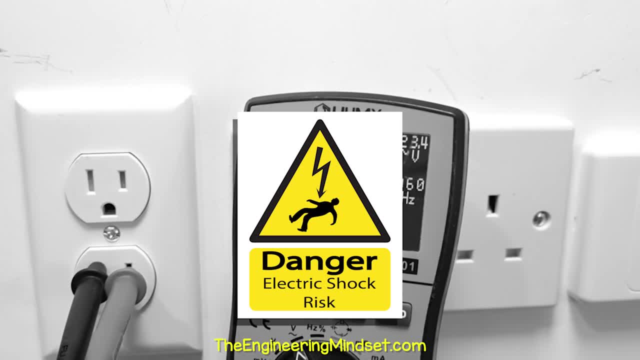 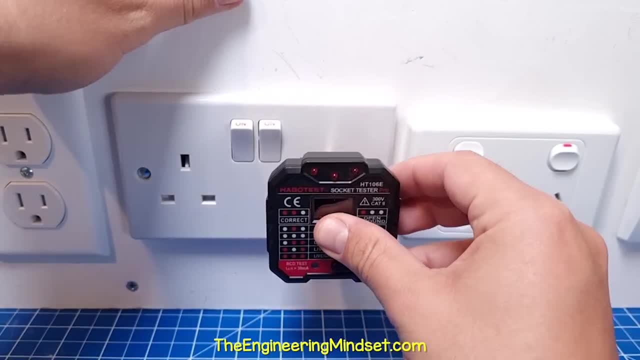 You should be qualified and competent to carry out any electrical work. You can buy socket testers which will test the wiring of your sockets. Some will even show you the voltage. These are much safer. I highly recommend that you use these devices instead. 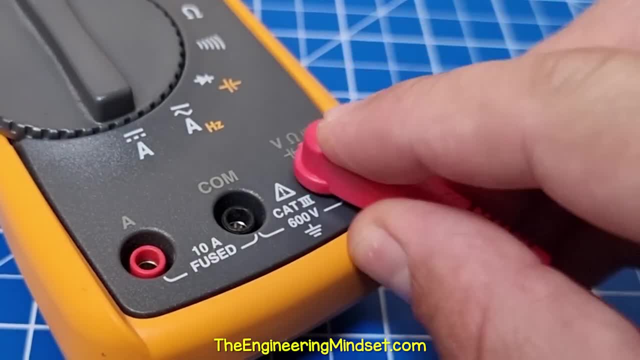 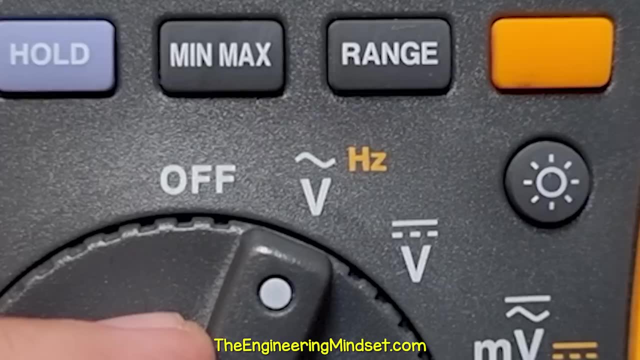 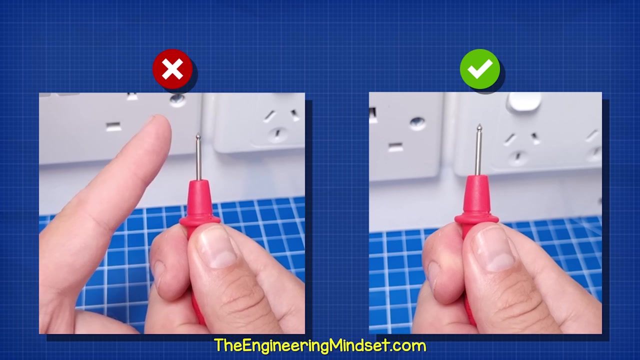 For AC voltage measurements, ensure that the red lead is in the V terminal and the black lead is in the COM terminal. On the auto range type, we simply select the AC voltage symbol. Keep your fingers away from the tips, as these will become electrified. If you touch this, electricity can flow through you and shock. 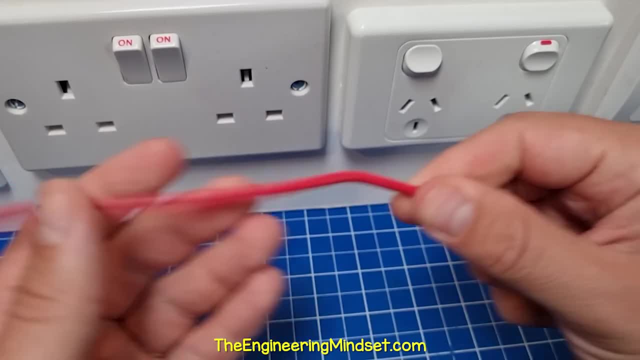 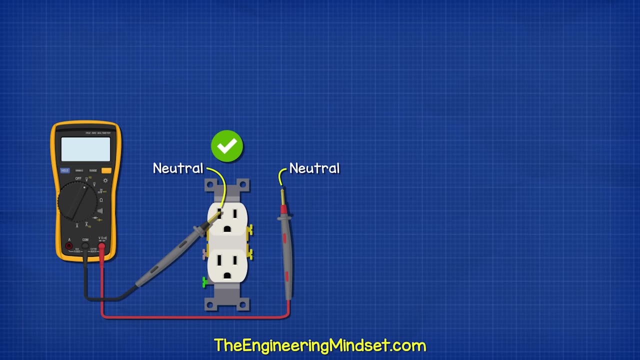 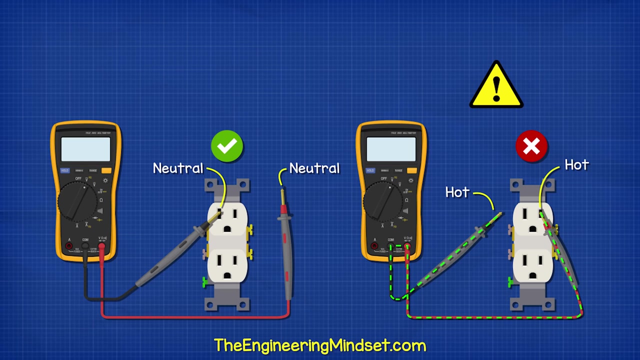 you Ensure the insulation on your cables is in perfect condition. Never use or try to repair a damaged cable, Just buy a new one. Always connect the black wire to the neutral first, because if you connect the red wire to an active terminal first, the black wire will instantly. 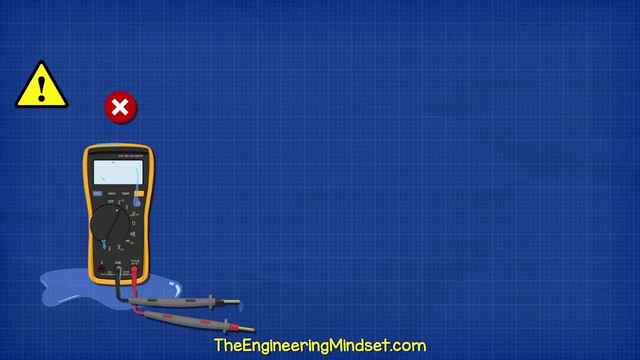 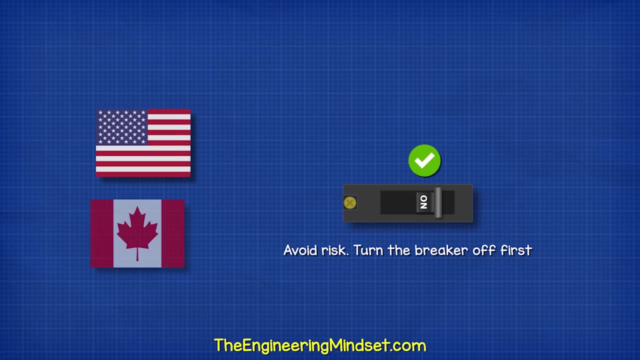 become electrified. If you connect the red wire to an active terminal first, the black wire will instantly become electrified. Do not use in wet conditions. wear rubber boots to insulate yourself and do not touch grounded surfaces. while taking measurements For North American circuits, I recommend you flip the breaker first. 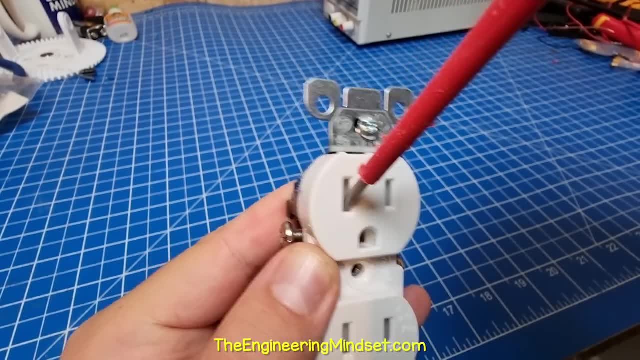 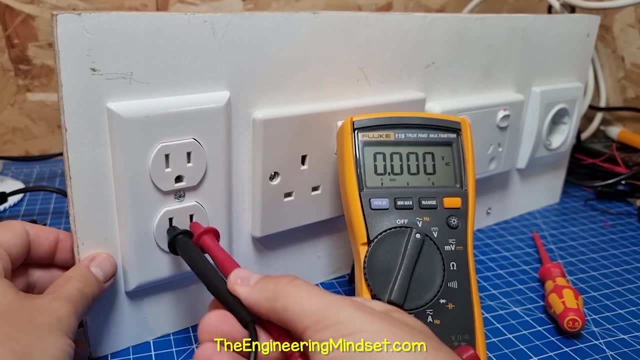 We often find a safety screen over the terminal of the socket, So we place the black probe into the large slot and the red probe into the small slot, and then we push until the safety screen opens When it is safe to do so. you may flip the breaker again and the meter. 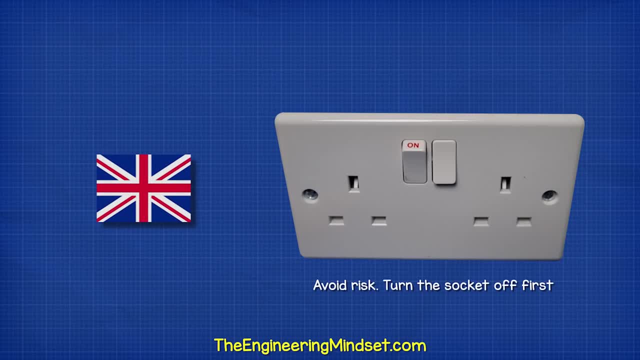 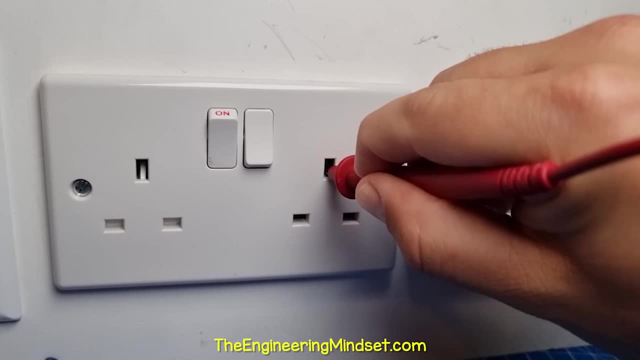 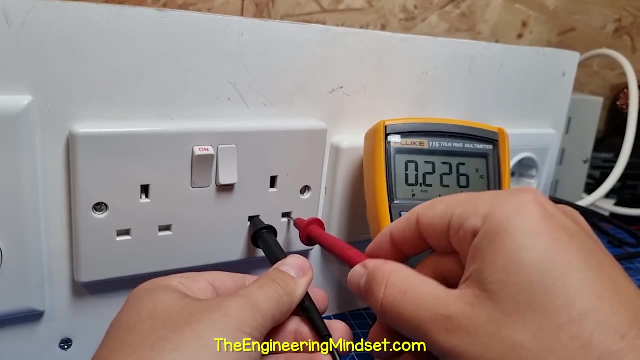 will then read the value For British circuits. turn the switch off first. We also have a safety screen on these types, so place the red probe into the earth terminal and push down to disable this. Then we place the black lead into the neutral terminal and the red lead into the live terminal. 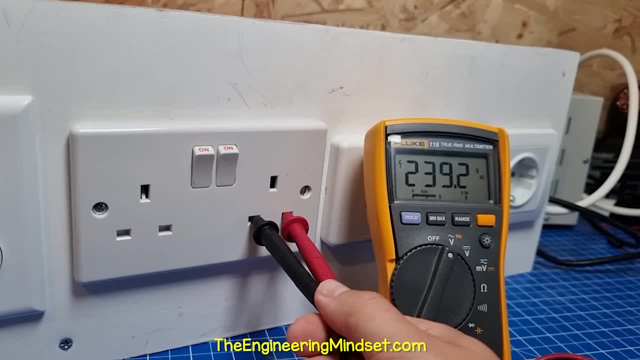 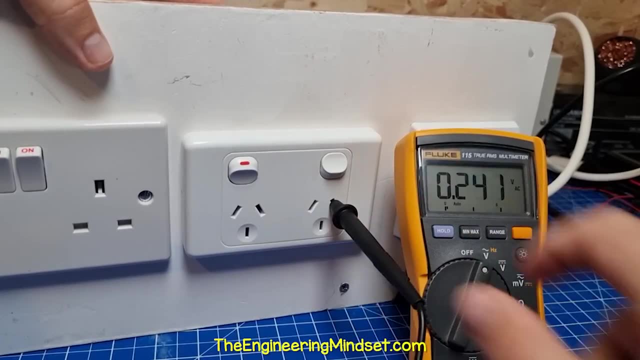 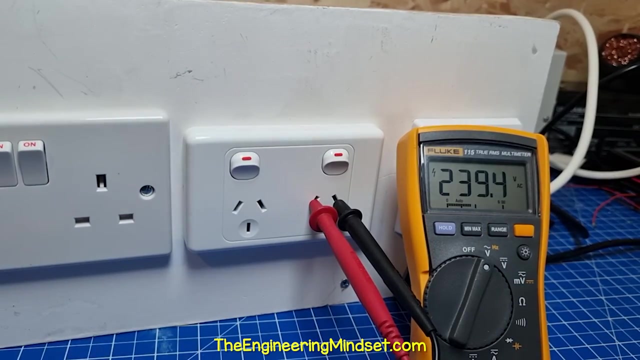 When safe to do so, flip the switch and the meter will then read the value For Australian circuits. turn the switch off first and then push the black probe into the neutral terminal and then the red probe into the active terminal. When safe to do so, flip the switch and the meter will then read the value. 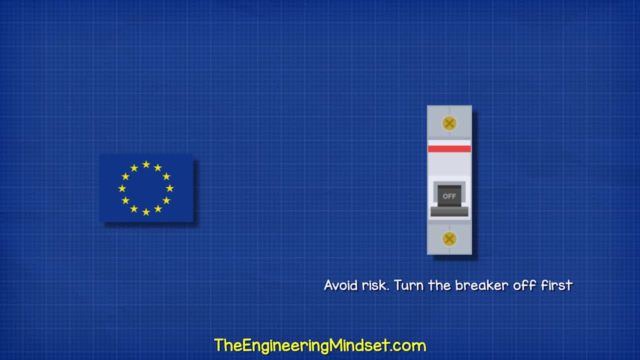 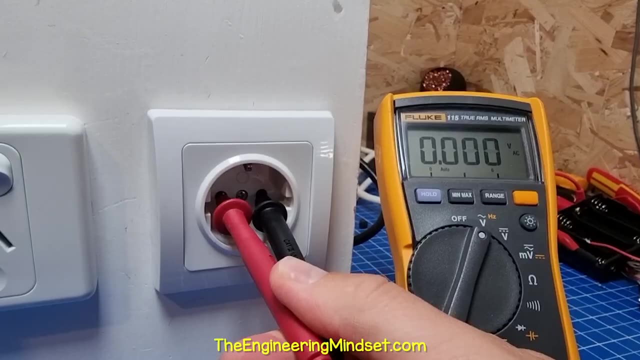 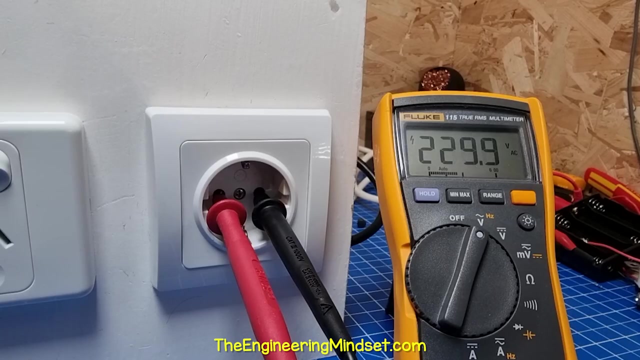 For European circuits. I would recommend that you first flip the breaker. We need to place the probes into the terminals and then apply a light pressure and tilt the leads to lift the safety screen, and then we can insert the terminals When safe to do so. we may then flip the breaker again. We can reverse the probes and see if there is a safety screen. If there is a safety screen, then we can insert the terminals When safe to do so. we may then flip the breaker again. We can reverse the probes and see if there is a safety screen, and then we can insert the terminals. 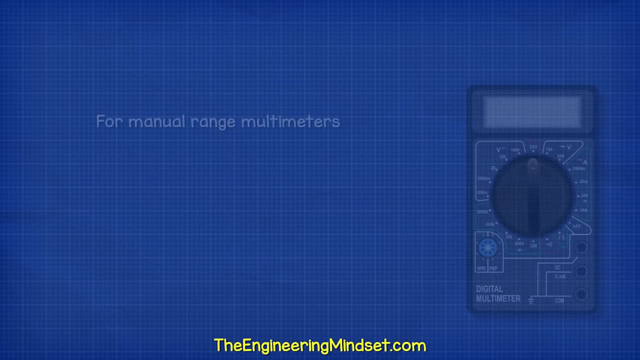 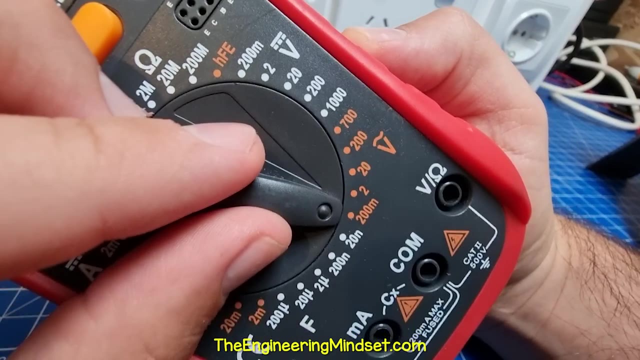 When safe to do so, we may then flip the breaker again. When safe to do so, we may then flip the breaker again. For manual range devices, we follow the same connection and safety procedures as the auto range tutorials, But on our meter we select the next value up from the voltage we are expecting to read. 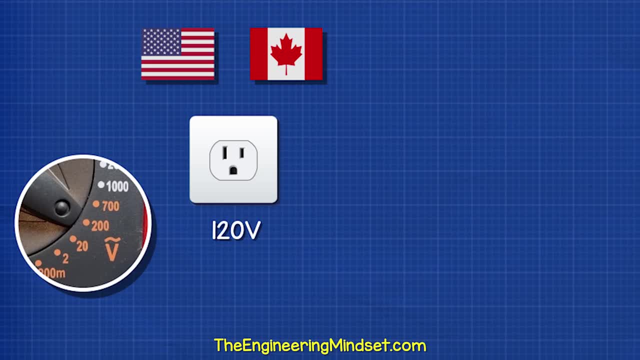 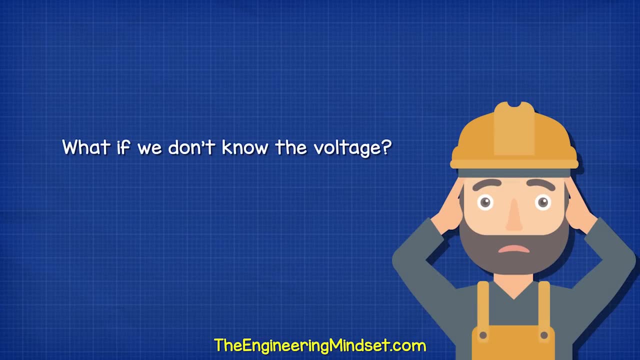 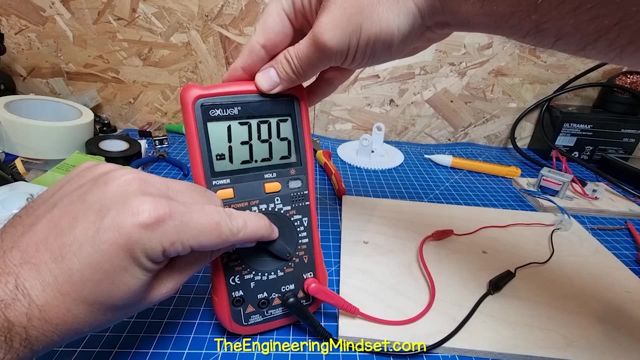 For example, on a 120V connection, we select the 200 setting. On a 230V connection, we select the 700 setting. If you are not sure of the voltage, start with the highest value first and turn the dial until the correct value is displayed. 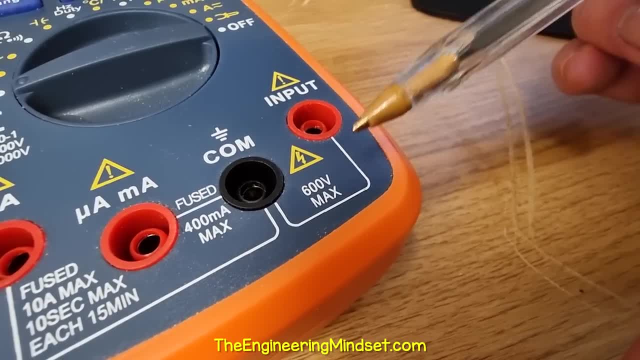 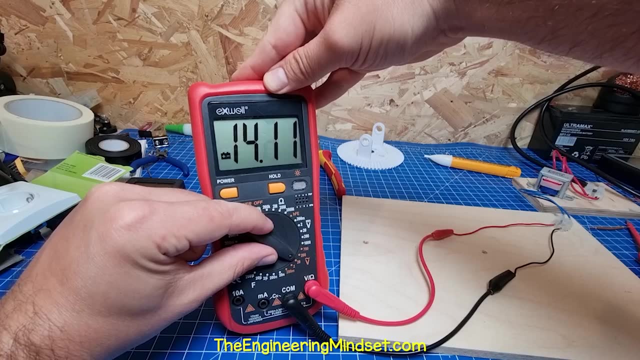 Do not exceed the maximum voltage of your meter. If the meter shows a 1,, the reading is out of range and you will need to turn the dial to a higher setting. You can buy either an average RMS or a true RMS multimeter. 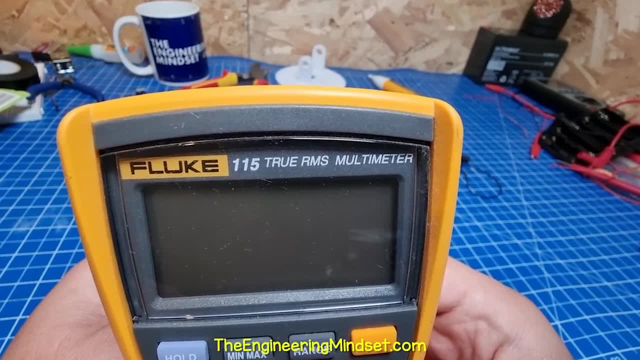 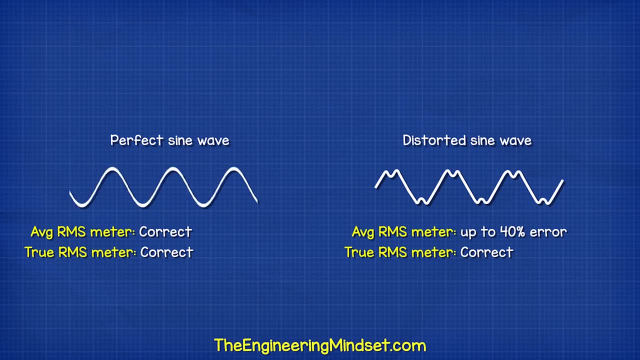 I'd highly recommend that you buy a true RMS type, as this is more accurate. Electrical equipment can distort the waveform. Only true RMS meters will accurately be able to measure this. Don't forget to check out PCBWay for all of your 3D printing. 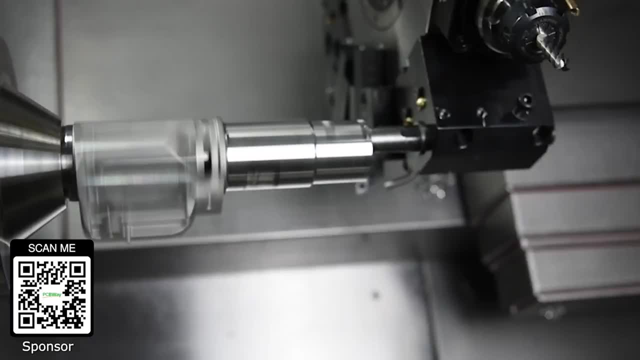 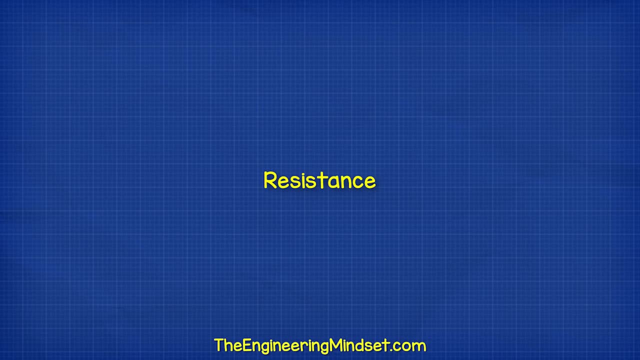 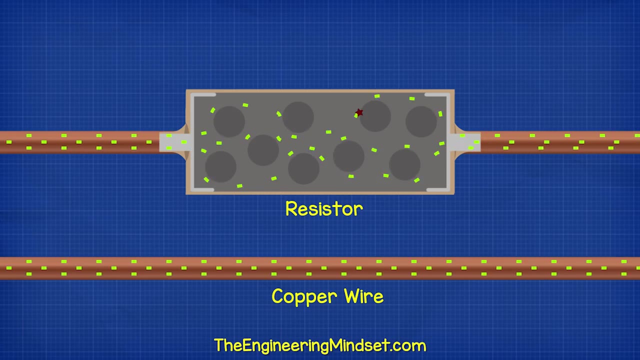 CNC machining, injection, molding and even sheet metal fabrication needs. I have a link for you in the video description down below. Resistance is represented by this symbol and it uses the unit of ohms. It's a measurement of how easily electrons or electricity 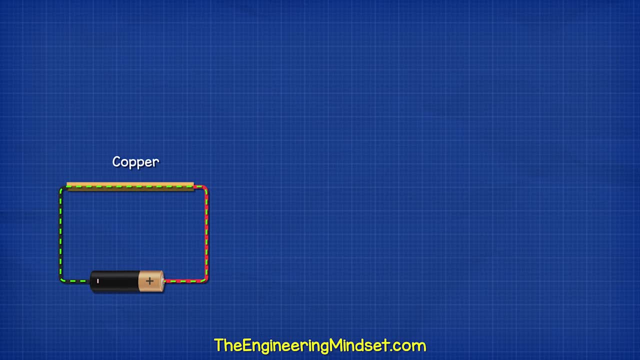 can flow through something. For example, electrons can flow very easily through this copper wire, Which is why we use copper wires. However, it's much harder for it to flow through this resistor And it's very, very difficult to flow through rubber. 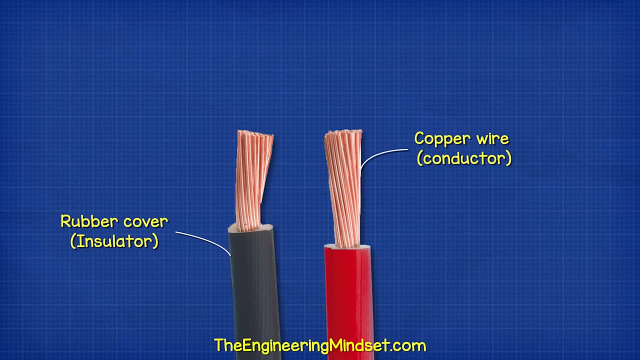 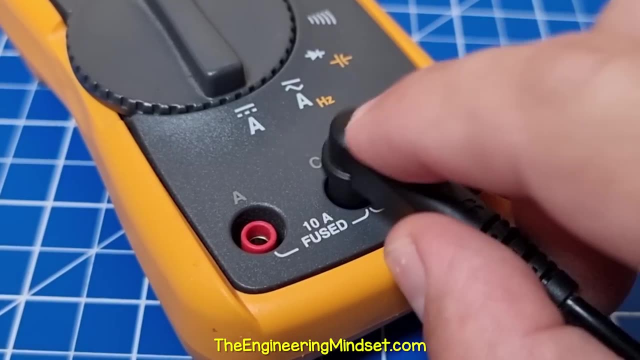 Which is why we use rubber insulation on the wires to protect us from the electricity in the copper wire. To measure resistance we need to place our black lead into the com terminal and the red lead into the terminal with the ohm symbol. 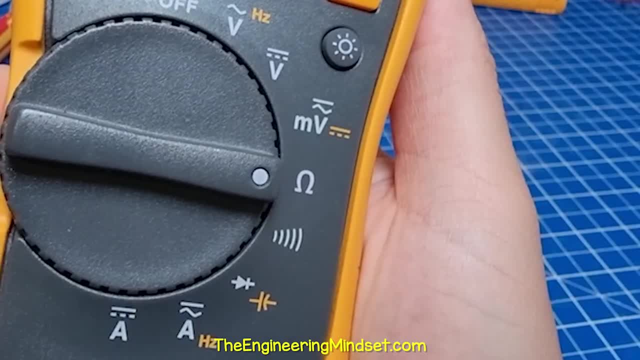 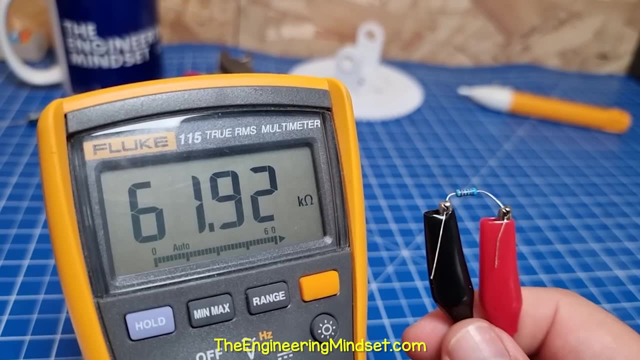 With the auto range device. simply turn the dial to the resistance setting and then connect your leads across the component. It doesn't matter which side you connect it. The device will now display the results. We can test items like speakers, resistors. 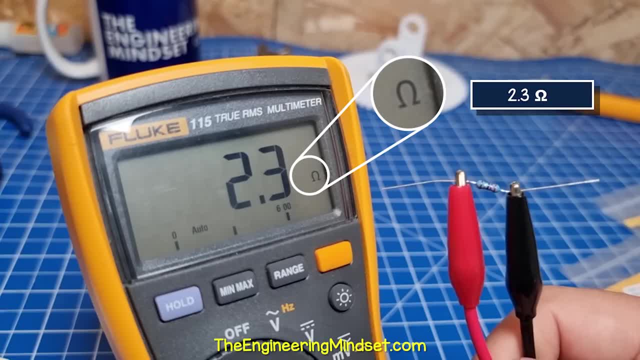 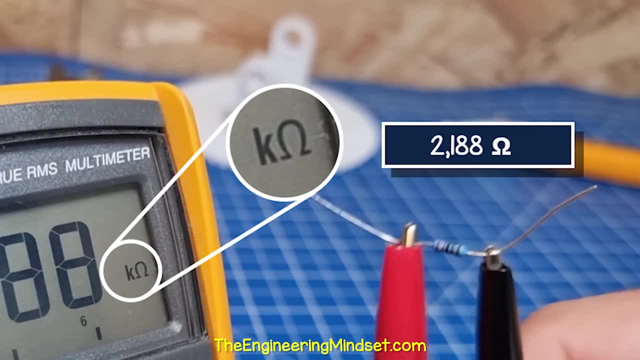 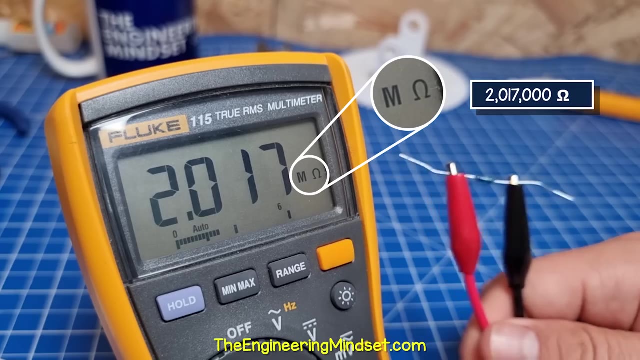 wires, potentiometers et cetera. But pay attention to the letters on screen. This one shows just ohms. This one shows k? ohms, meaning 1,000 ohms. This one shows m ohms, meaning mega or million ohms. 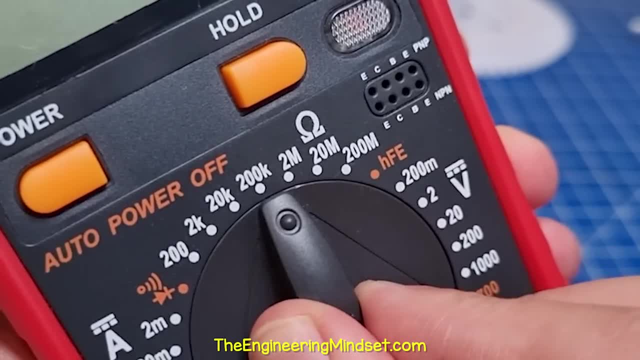 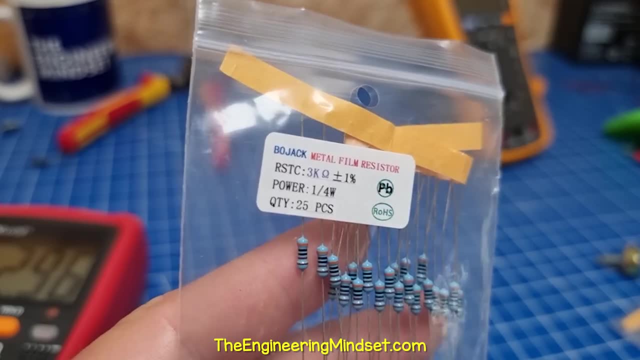 With the manual range. we need to select the correct setting. Remember we use the next number up. For example, this resistor is rated at 3k ohm. That's more than 2k, so we go to the next value up. 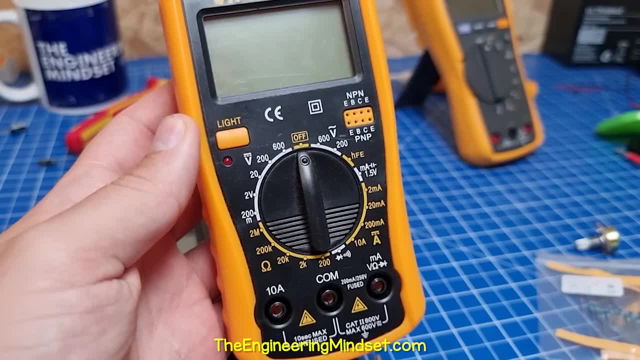 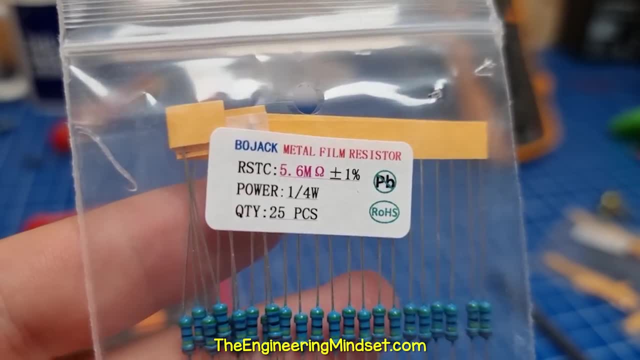 which is the 20k, and then we can see the result. This multimeter has a maximum setting of 2 ohms. So if I try to read this 5.6m resistor, it will just show a 1, because it's unable to measure values this large. 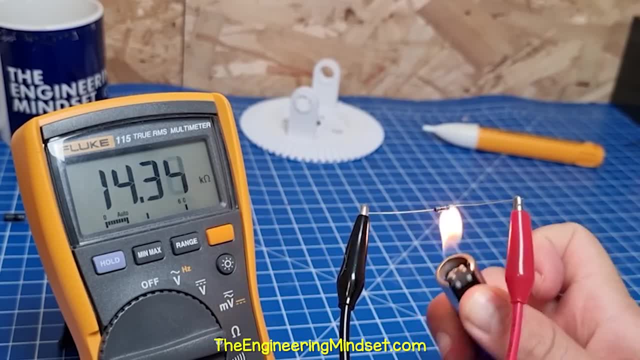 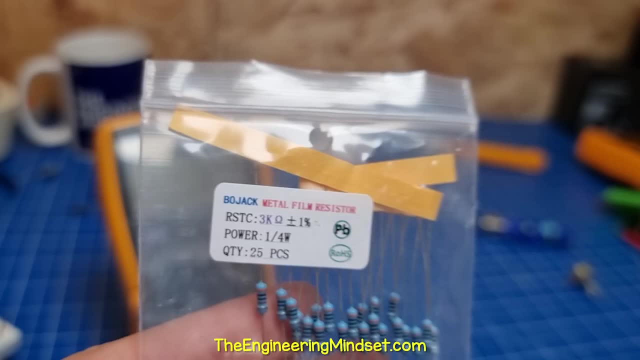 Do be aware that the resistance also changes with temperature. Resistors also have a tolerance. This one shows 3k ohms plus or minus 1%, So it could be anywhere from 3030 ohms to 2970 ohms. 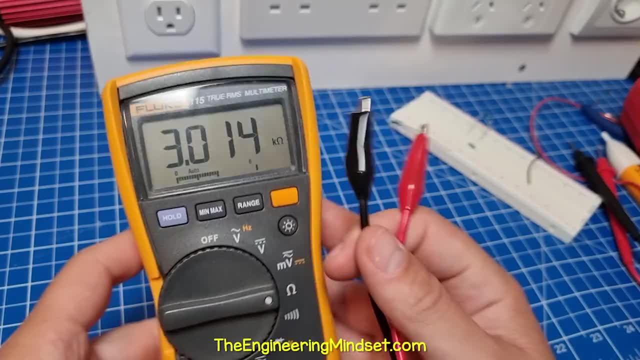 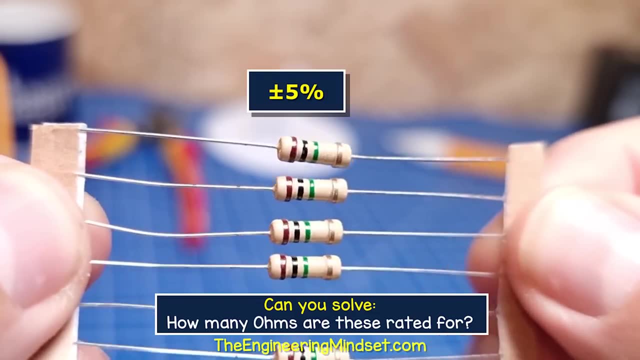 So it could be anywhere from 3030 ohms to 2970 ohms, But when we measure it it's 3014 ohms, So this is within the stated tolerance. Other resistors like this one have a 5% tolerance. 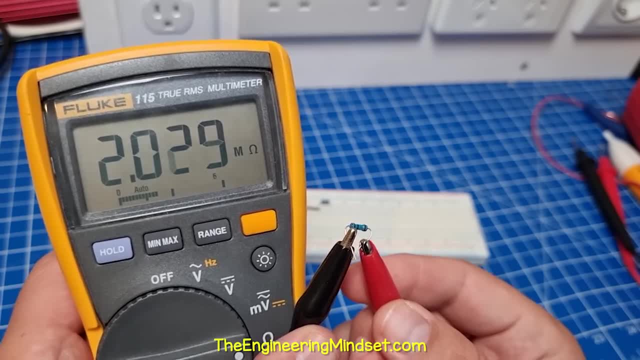 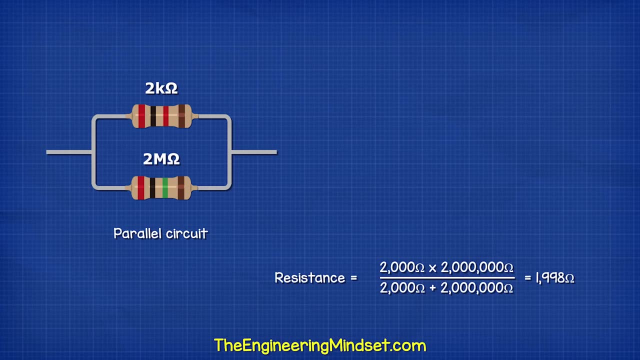 However, this resistor is around 2 mega ohms, But when we add it to this simple circuit, we get a reading of around 2 kilo ohms. That's because it's now in parallel and resistance divides, So do not try to test components on a circuit board. 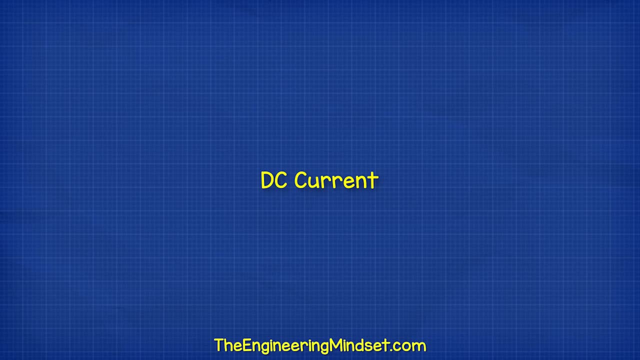 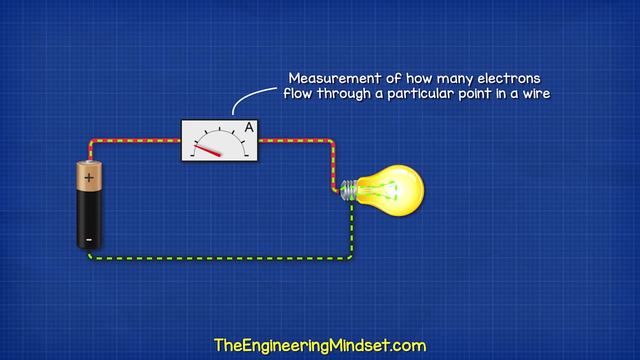 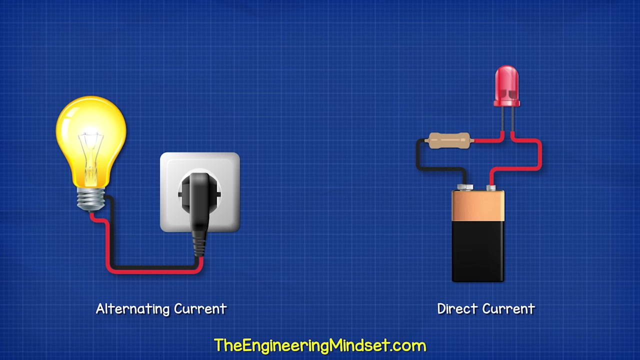 without isolating them first. Current is a measurement of how many electrons are flowing through a particular point in a wire. Direct current means the electrons flow in just one direction. We typically find this in battery operated equipment. It is measured in amps or amperes. 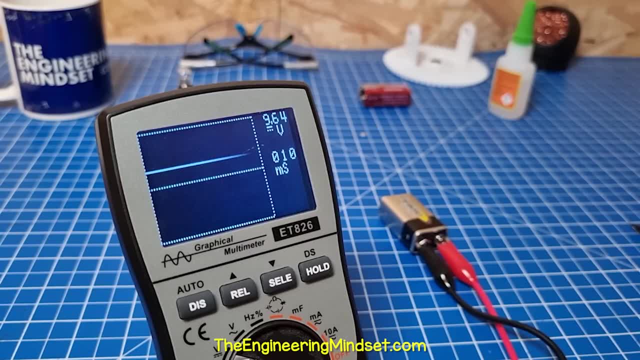 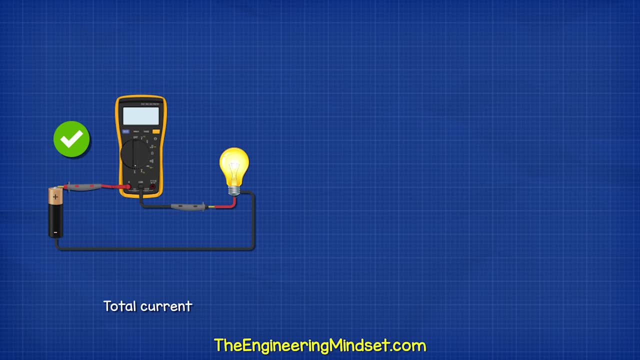 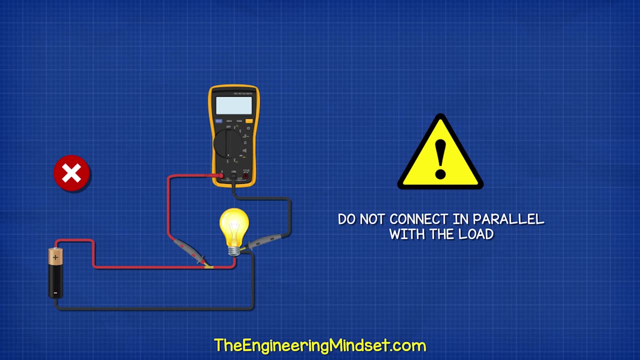 This uses the symbol A. The dash line just represents direct current. We must place the multimeter in series with the circuit And we can do this either for the total circuit current or the branches of the circuit. Do not connect the meter in parallel with the load. 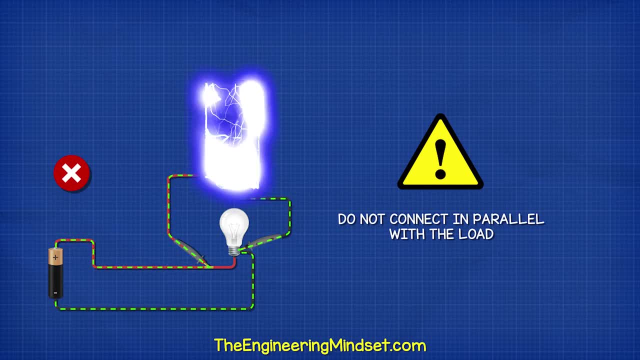 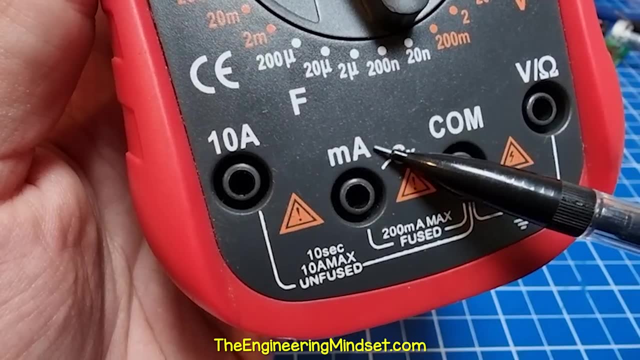 This can cause a large current to flow through your meter and it will damage it. Your meter will either have three or four terminals. One of them will likely show MA or milliamps. It should also state a number to indicate the maximum milliamp current. 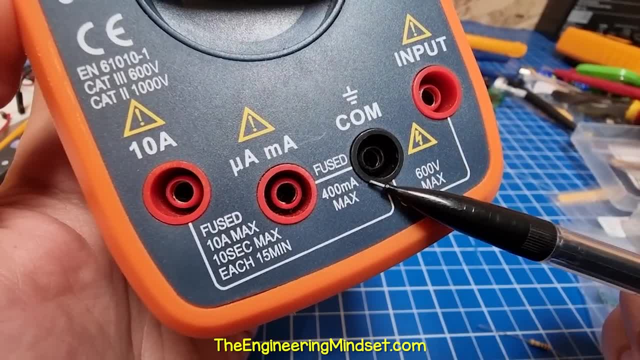 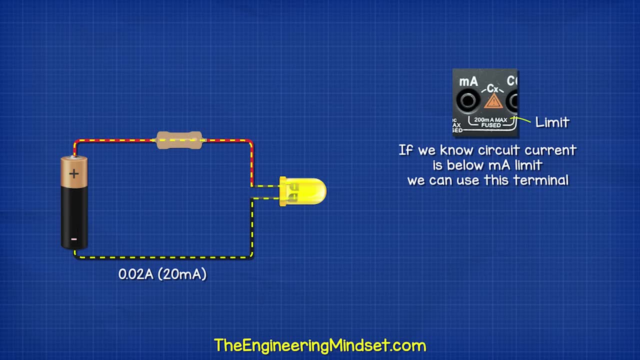 that it can measure through this terminal. This one, for example, states a maximum of 400 milliamps. If we know the circuit that we're testing is below this, we can place the red lead into this terminal. Otherwise, we must use the A terminal. 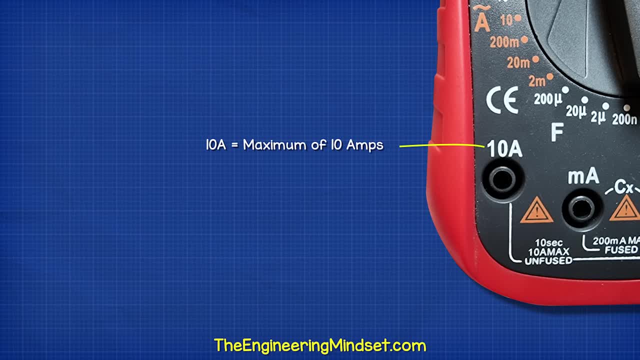 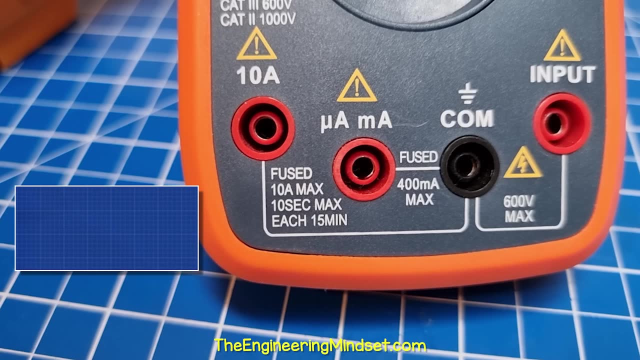 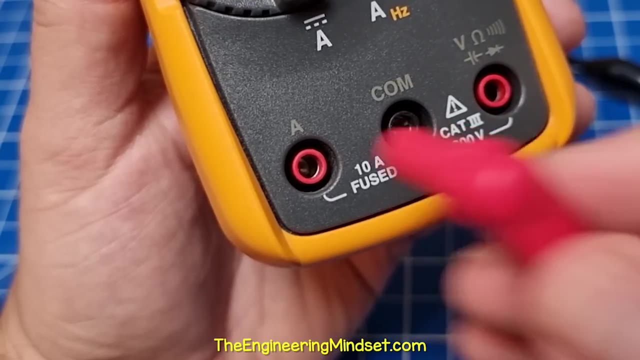 This is usually stated as 10A, meaning a maximum of 10 amps. The time indicates for how long it can be connected for, For example, 10 amps for 10 seconds per 15 minutes. Now select the direct current setting and place your red probe into the 10A terminal. 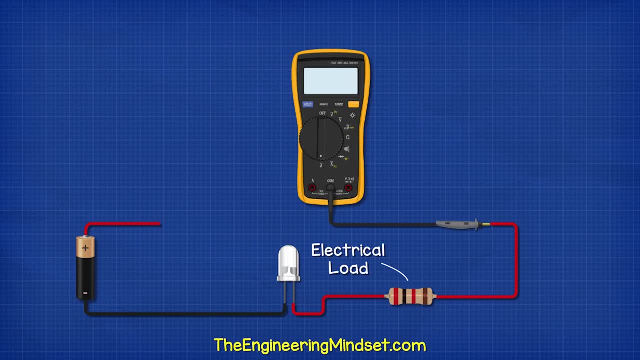 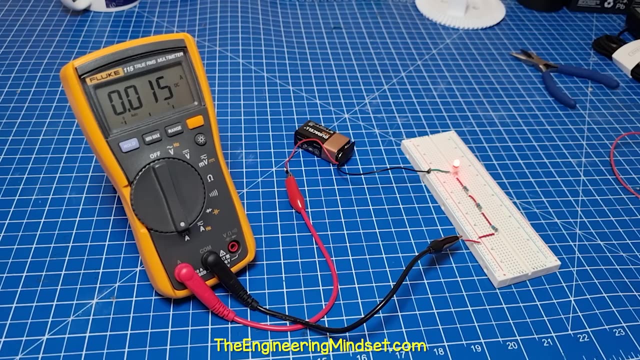 and the black lead into the COM terminal, Connect the black probe to the load side and the red probe to the supply side, And then ensure that the multimeter is in series with the circuit. Once the circuit is powered, we will then get the result. 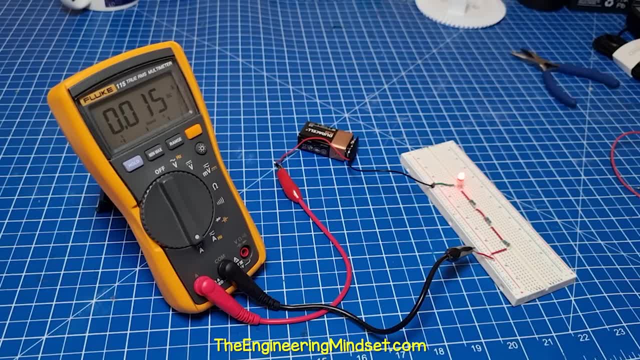 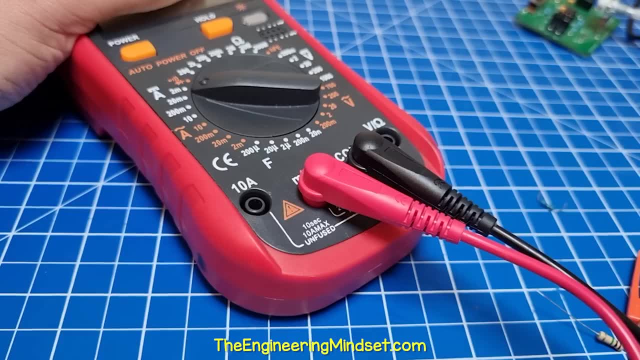 With the manual range. we need to select the correct setting. We already know that this circuit is around 15 milliamps, So we use the milliamp terminal and then choose the next terminal. We select the next highest value, which in this case is 20 milliamps. 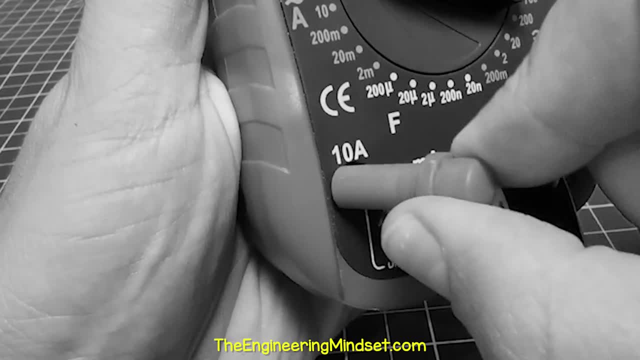 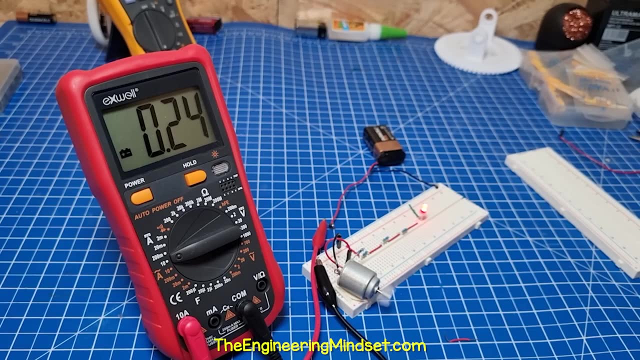 We can then see the result. If we do not know the current, then we start by using the 10A terminal, We select the highest setting and we work our way down, Although here it shows it's just 0.25 amps. 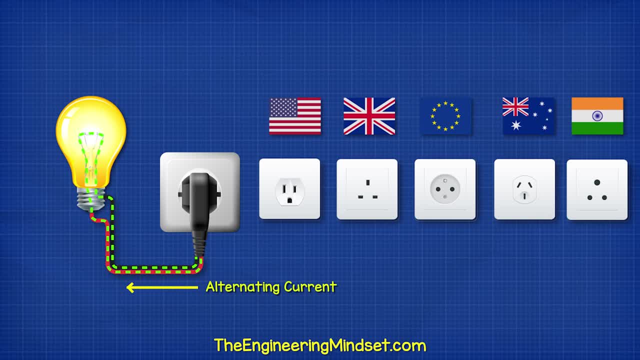 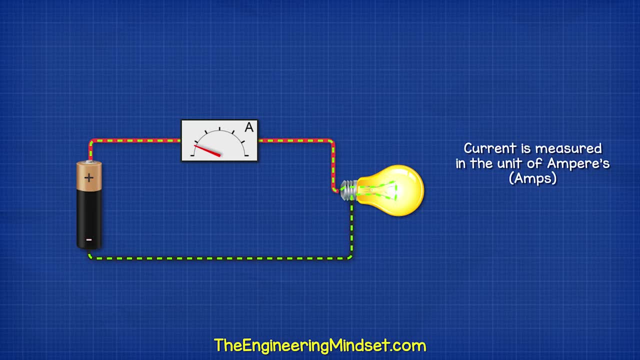 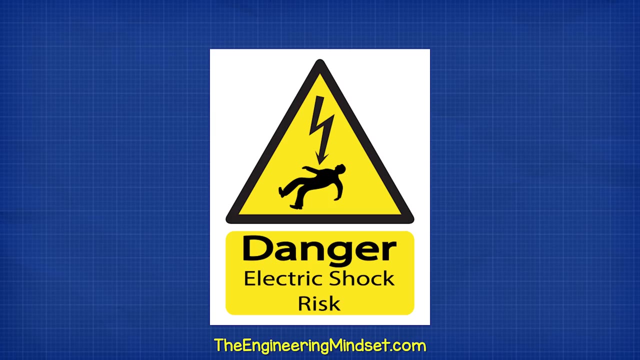 Alternating current means. the electrons in the electrical system are constantly flowing backwards and forwards. We find this in our home's electrical system. It is measured in amps or amperes. This is represented by the letter A with a sine wave. Remember, electricity is dangerous and can be fatal. 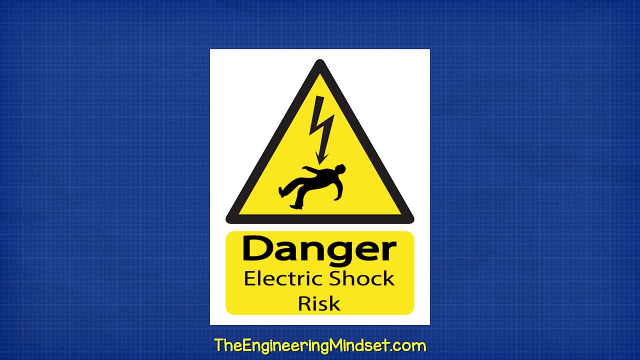 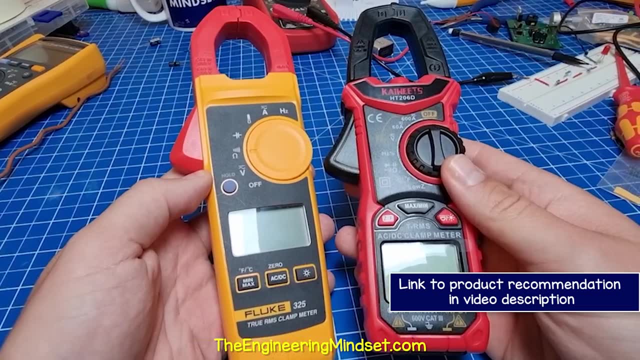 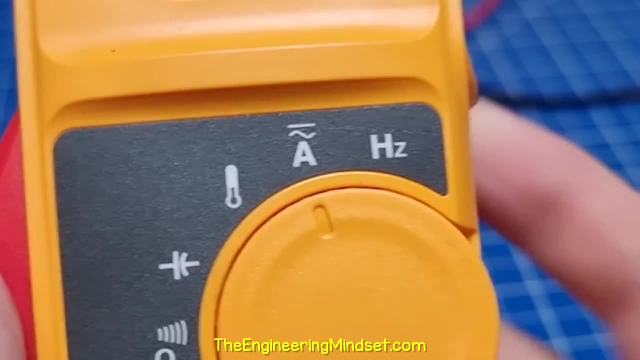 You should be qualified and competent to carry out any electrical work. If you just need to measure AC current through a wire, I would highly recommend that you instead use a clamp meter. This is much safer. Simply clamp around one wire and select the alternating current option. 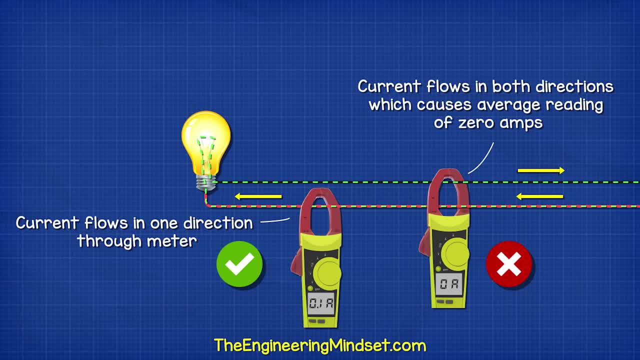 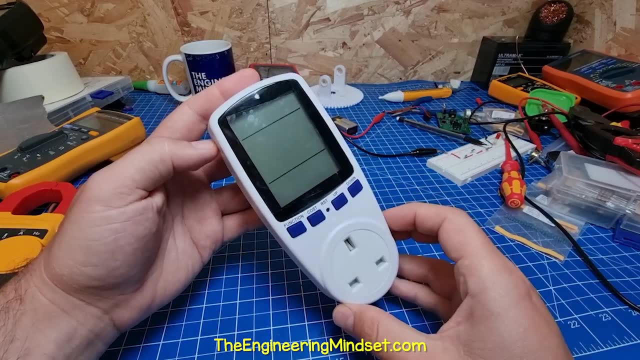 If you clamp the active and neutral wires together, the current will cancel each other out and you will not get an accurate reading. If you need to measure the current of a device, then just buy an energy monitor plug instead and plug your device into this. 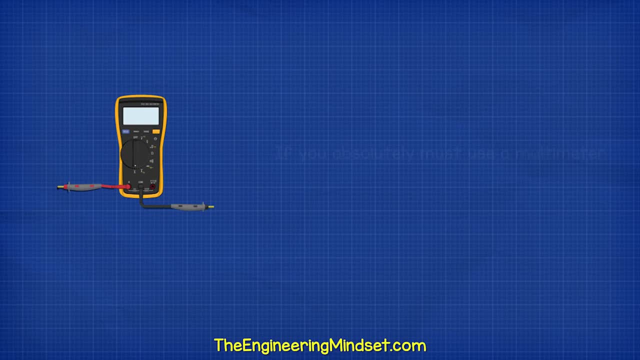 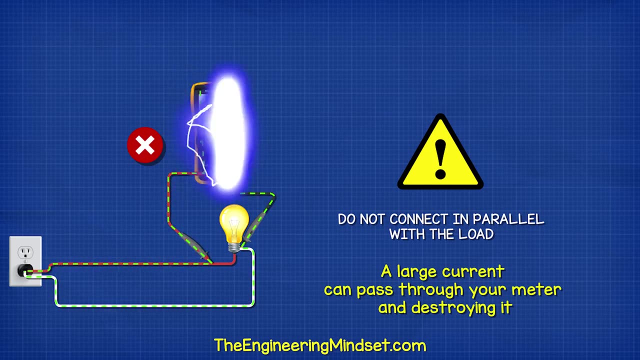 It will safely show you the current voltage and power. If you absolutely must use a multimeter, then we have to connect the device in series with the circuit. The device has a very low internal resistance, so connecting in parallel will expose the meter. 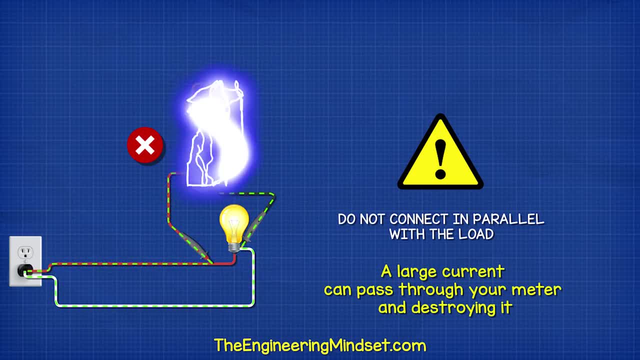 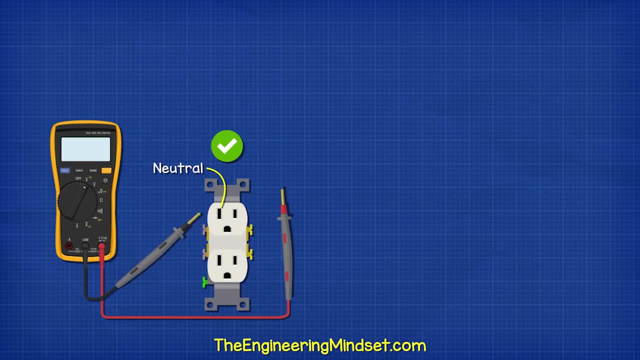 to the full voltage of the circuit and this will instantly cause an enormous flow of current through your meter and it will destroy it. So be very careful. The probes will also become electrified along with any conductive surface they come into contact with. 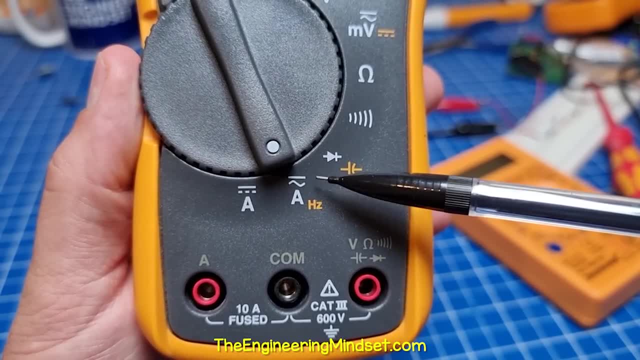 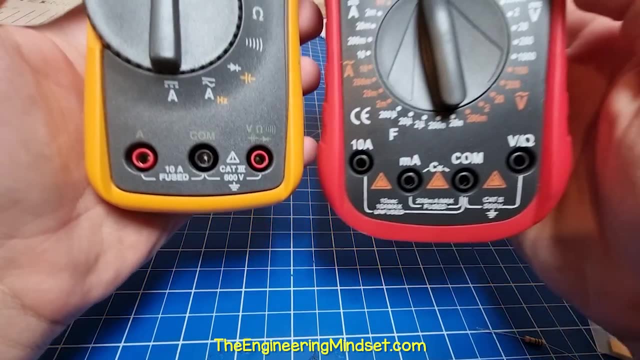 Again, be careful. First check that your meter has an AC current setting. If it doesn't, then do not attempt to use it for this purpose. Next, check the terminal identification. Some will have a dedicated terminal for measuring milliamps. 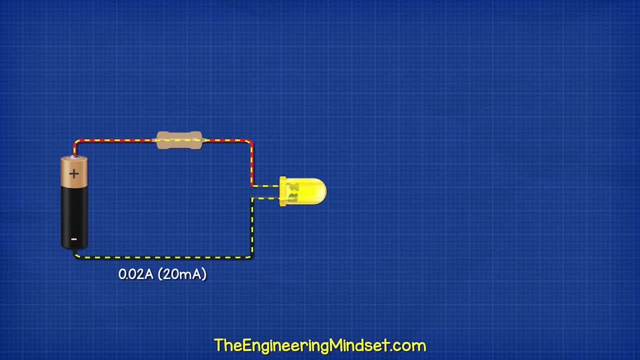 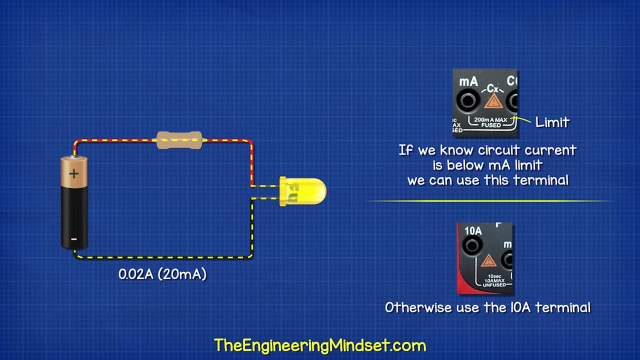 and it will state the maximum current that it can handle. If you know that your circuit will exceed this or you do not know the maximum current, then we need to use the terminal marked with an A. Typically, this will be labeled 10A. 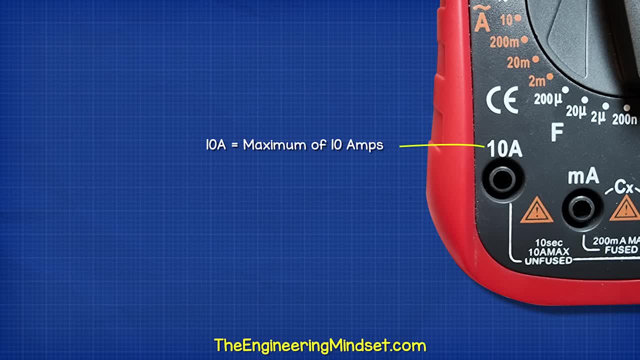 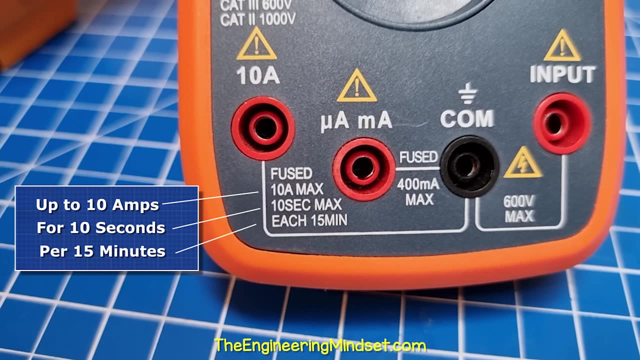 indicating a maximum of 10 amps can be connected. It usually tells you for how long, for example, a maximum of 10 amps. for example, a maximum of 10 amps for 10 seconds, and you must then disconnect it for 15 minutes to cool down. 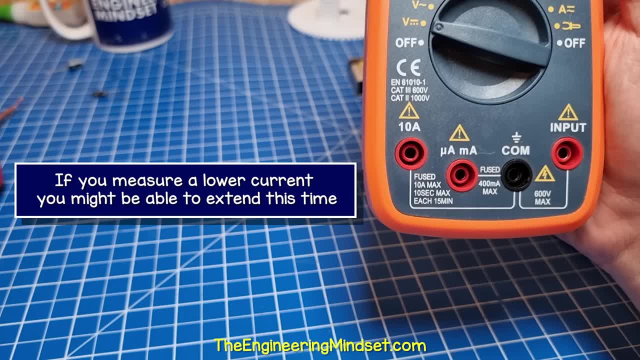 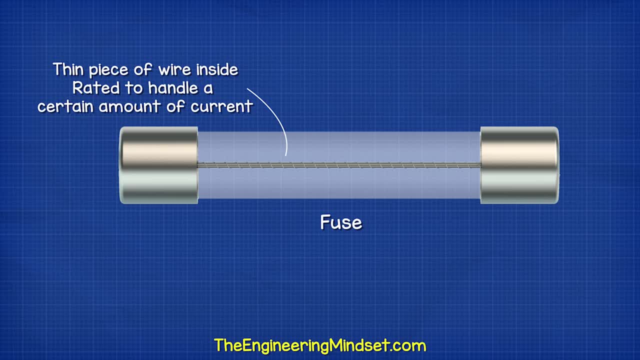 If you measure a lower current, you might be able to extend this time. Please check the manufacturer's guide for this. Most meters will come with a fuse to protect the device. This heats up and breaks the circuit if you exceed 10 amps. 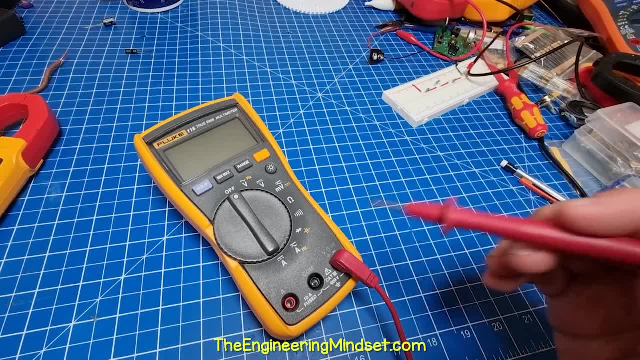 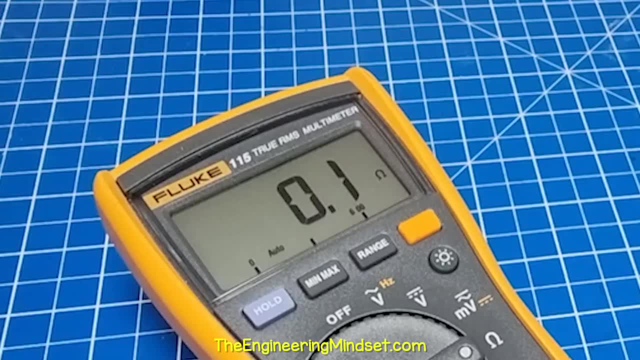 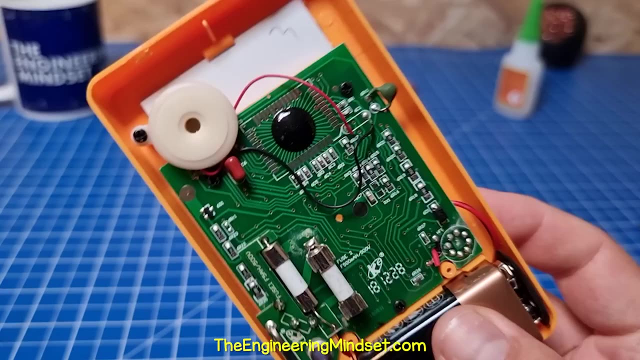 You can check the fuse by connecting the red lead to the V terminal and placing the probe into the fuse terminal, and then we select the resistance setting. If it states a value of less than 0.5, it should be okay. If it states OL, then it is broken. 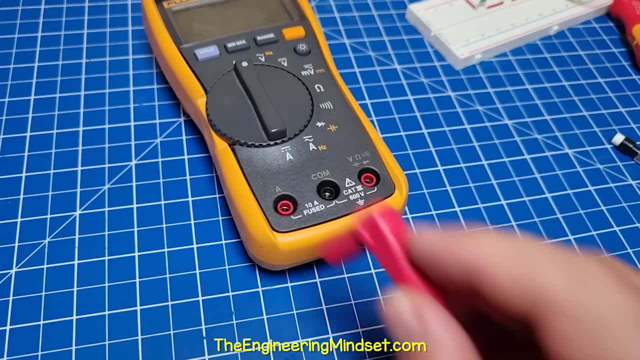 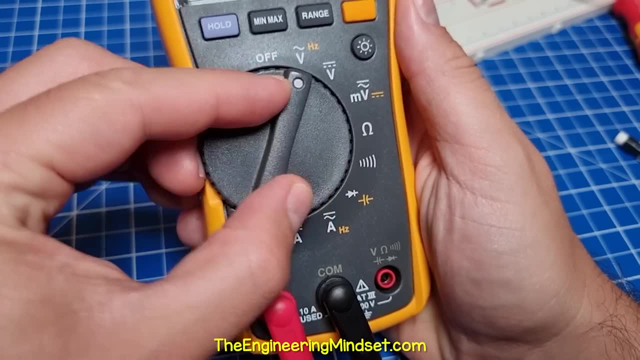 You can remove the back cover to replace the fuse. To use the multimeter, place your red probe into the 10A terminal and the black lead into the COM terminal and then select the alternating current setting. Ensure the power is disconnected from the circuit. 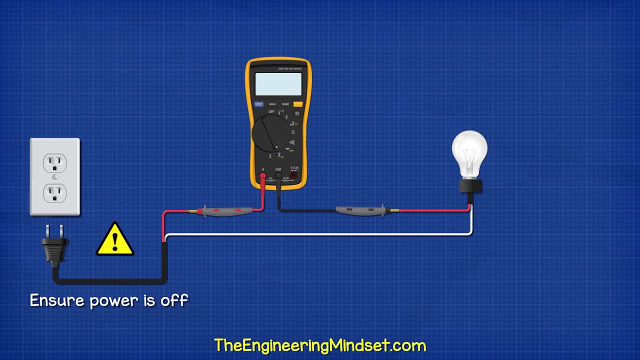 Connect the black probe to the load side and the red probe to the supply side, ensuring your meter is now in series with the circuit. Check the area and ensure it is safe to turn the power back on. You will then see the results If you have a manual range meter. 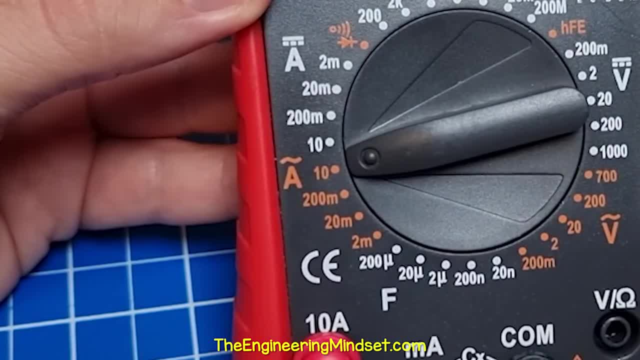 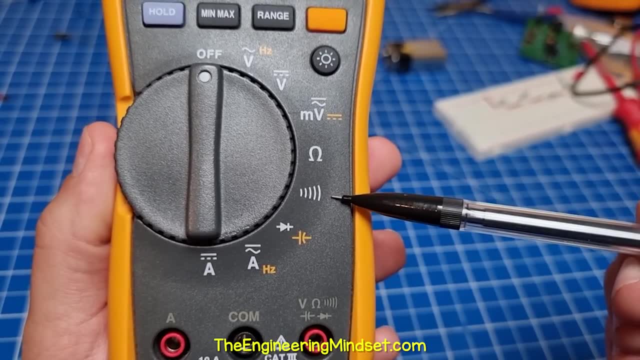 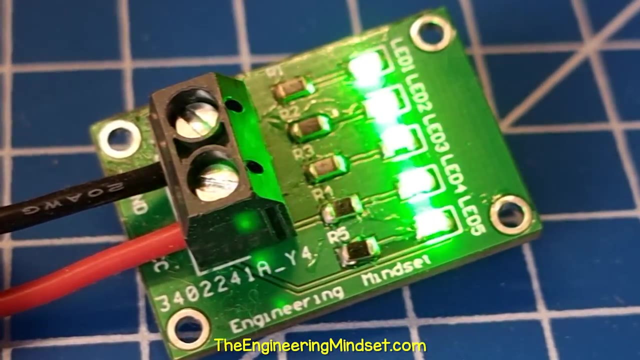 start with the highest setting. This is usually 10 amps. It will then display the results. We use the continuity function to test if two points in a circuit are connected. If so, it means electricity can flow. Simply connect your black lead into the COM terminal. 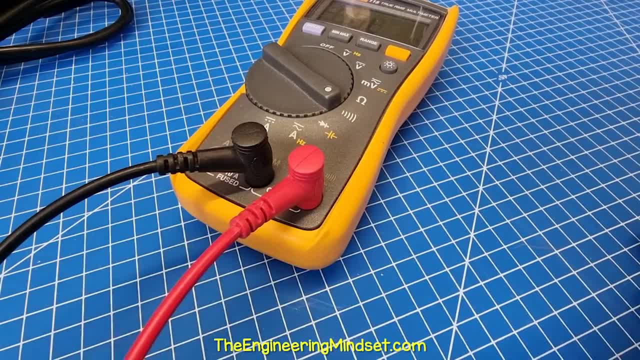 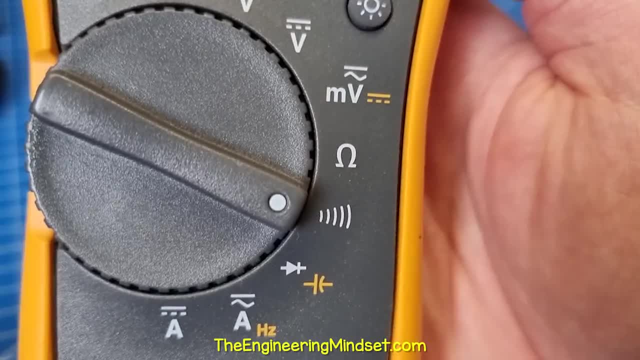 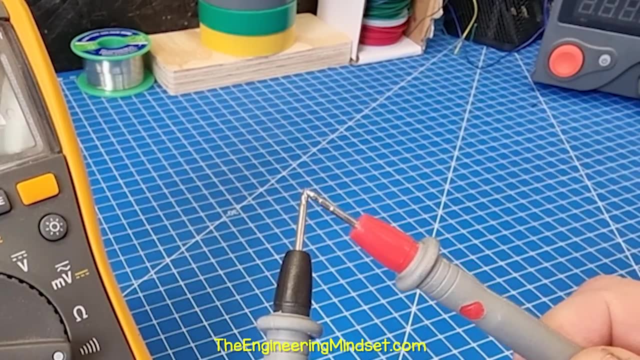 and the red lead into the terminal with the continuity symbol. If it doesn't show this, but it has the function, then we can use the V terminal. The screen will default to OL, meaning open loop. Tap the leads together to test the meter. 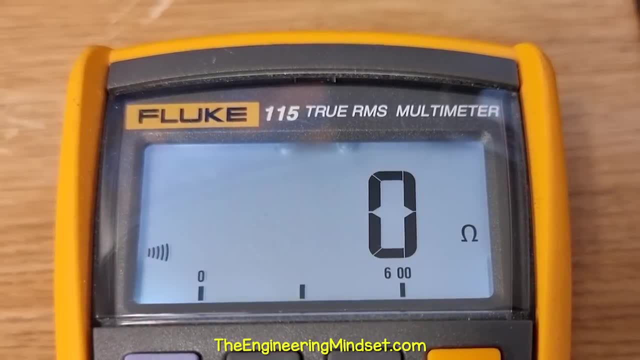 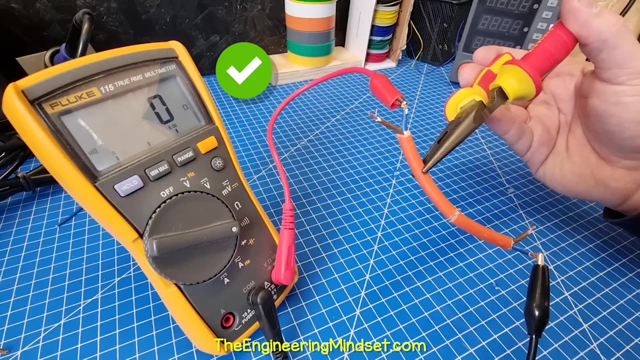 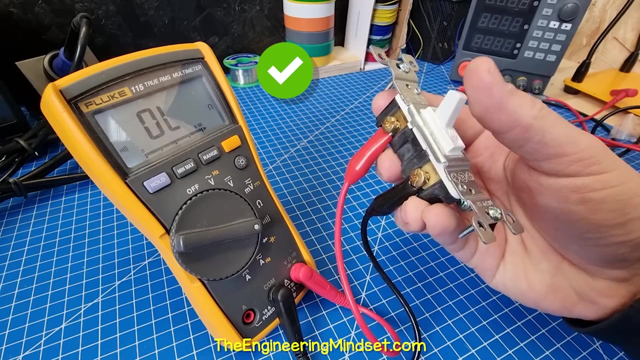 You should hear a continuous tone. It will also display the resistance. Usually in wires this is around zero ohms or very close. We can use this setting to test a break in the circuit or a wire. We can test that switches operate correctly. 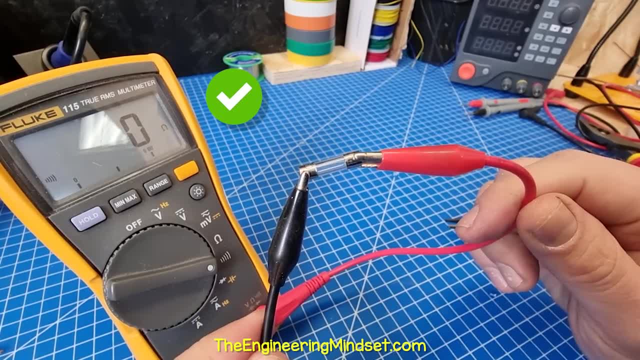 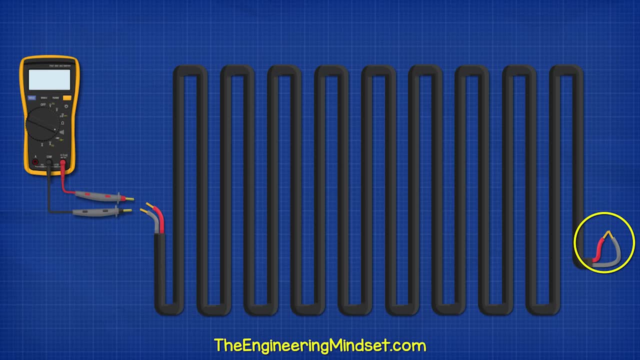 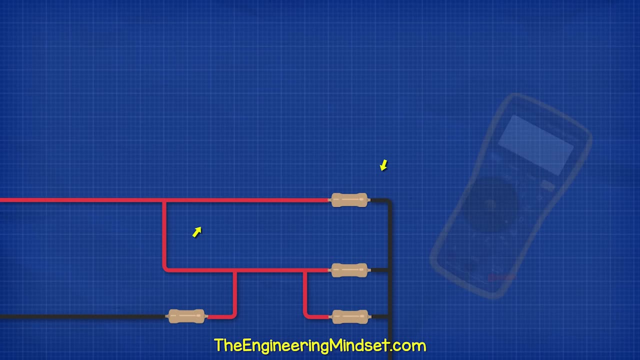 and we can check if fuses are also working correctly. We can test cables over very long distances by connecting one end together and testing the other end. It's important to know that we can get false readings, though, If we try to test between these. 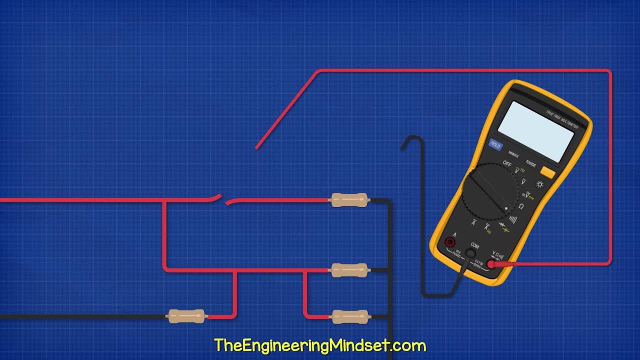 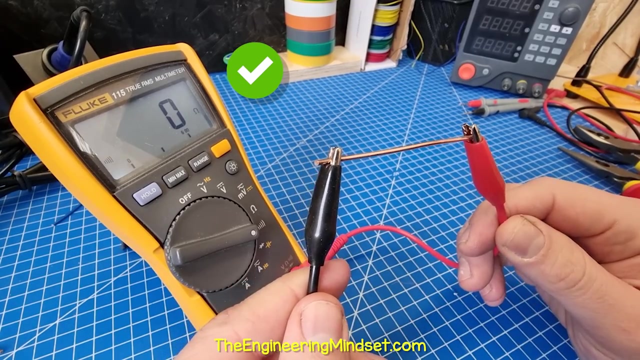 these two points which are clearly broken. the meter has found an alternative route, and so it will indicate continuity. You must consider this and isolate where possible. Continuity tests do not work with high resistance circuits, For example. this wire is fine. 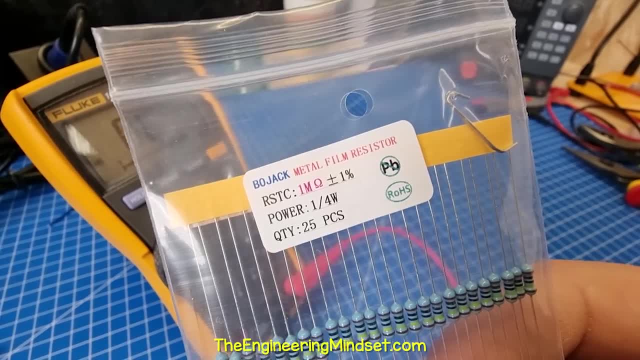 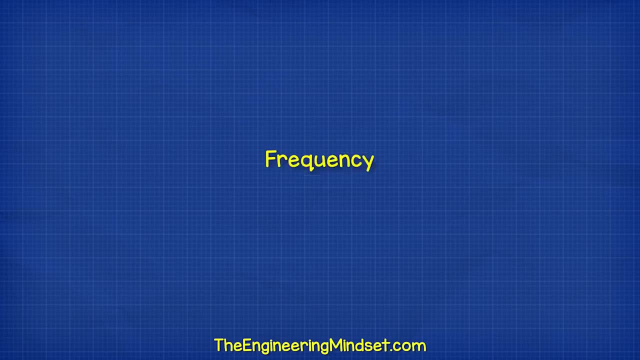 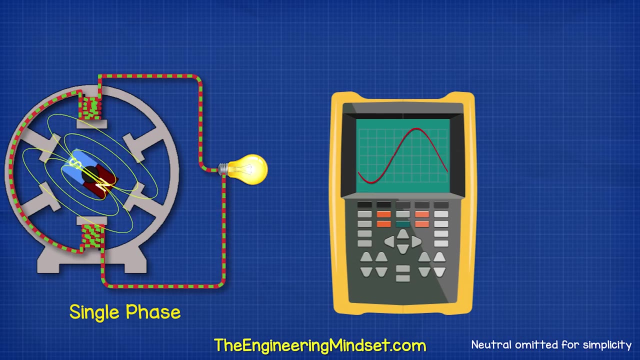 This low value resistor is also fine, but this high value resistor is too much and the meter indicates that there isn't continuity, even though there is. Frequency uses this symbol. This refers to how many times the pattern of an electrical signal repeats per second. 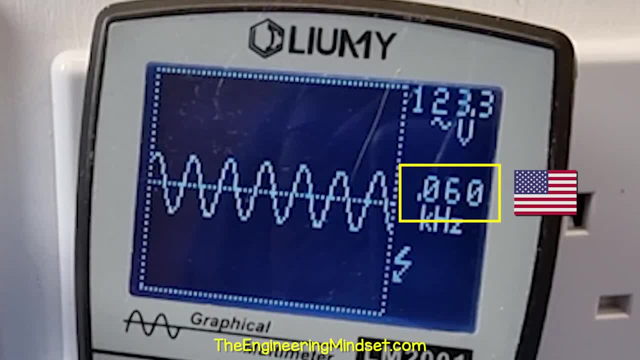 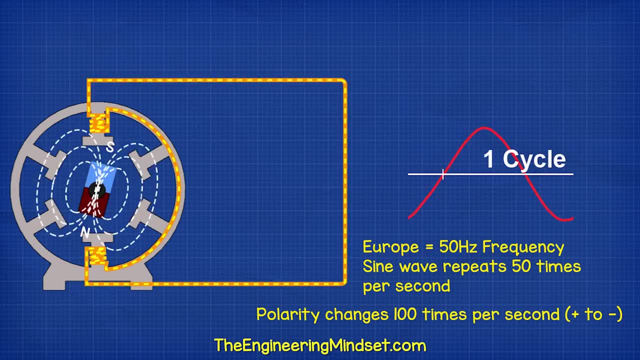 For example, homes in North America use 60 hertz and homes in Europe use 50 hertz. This just means that the AC sine wave repeats 60 or 50 times per second, but we measure this in the unit of hertz. 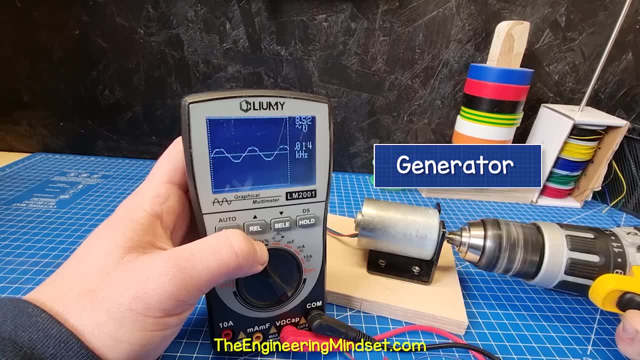 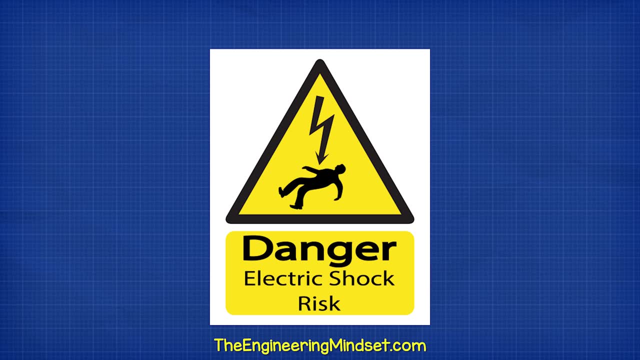 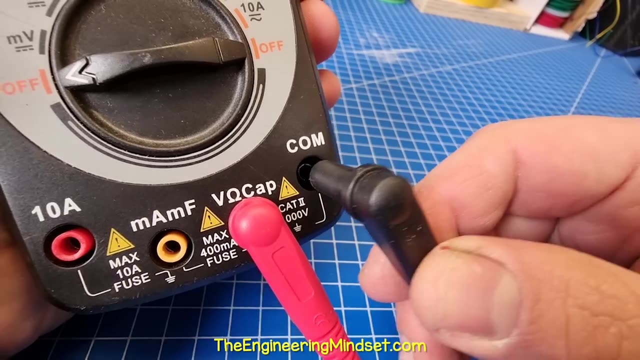 This is all to do with the speed of the electrical generator. Remember, electricity is dangerous and can be fatal. You should be qualified and competent to carry out any electrical work. To read frequency, we insert the red lead into the V terminal and the black lead into the COM terminal. 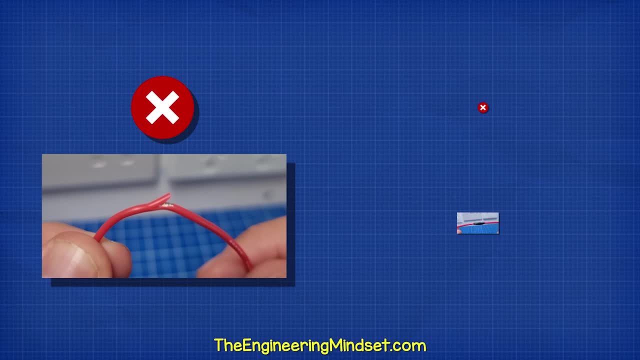 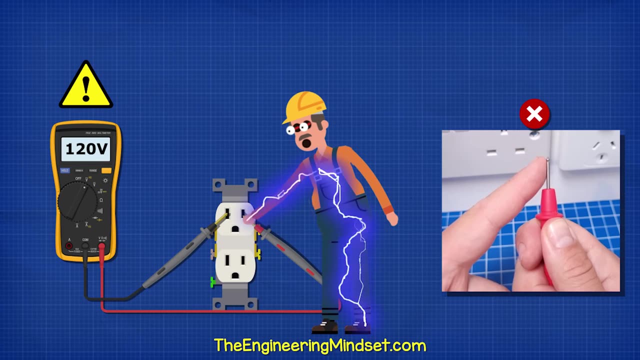 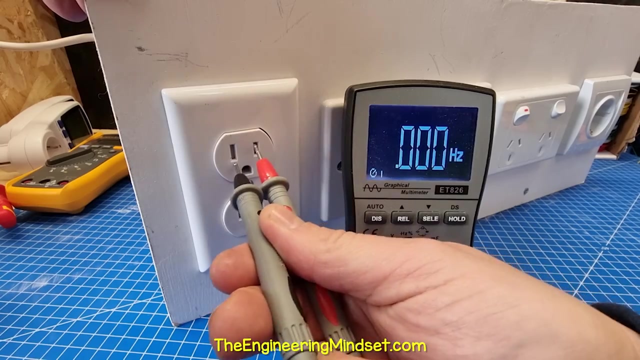 then select the frequency function on the meter. Ensure your leads, equipment and working area is safe, and I recommend turning the power off first. Do not touch the probe ends, wear rubber boots to insulate yourself and stay away from any grounded surfaces. 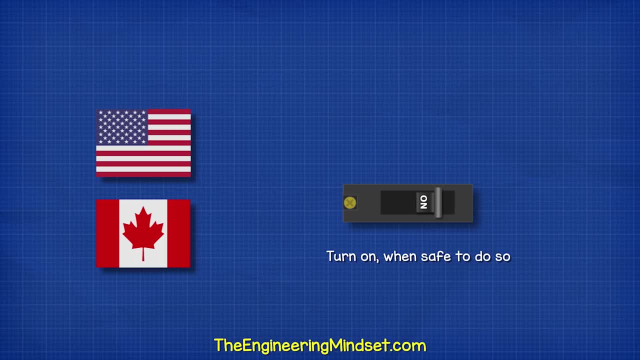 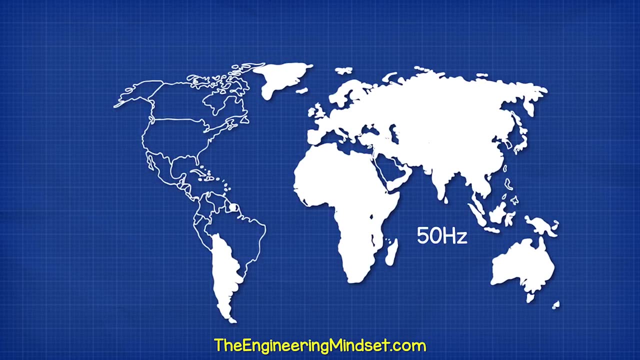 Then connect into the electrical system and, when it is safe to do so, turn the power on. The meter will now show the frequency and the value will change depending on where you are in the world. Turn the power off before disconnecting. 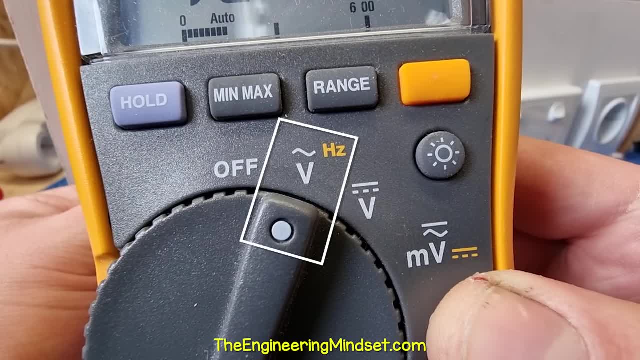 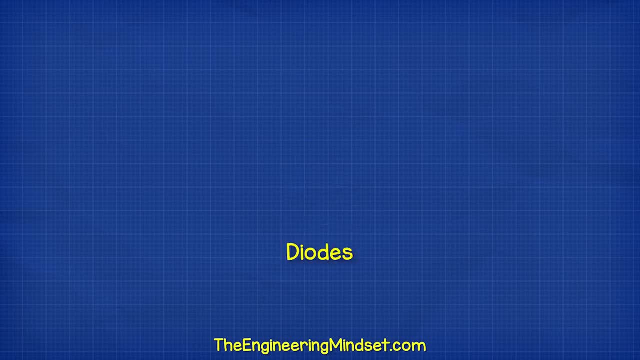 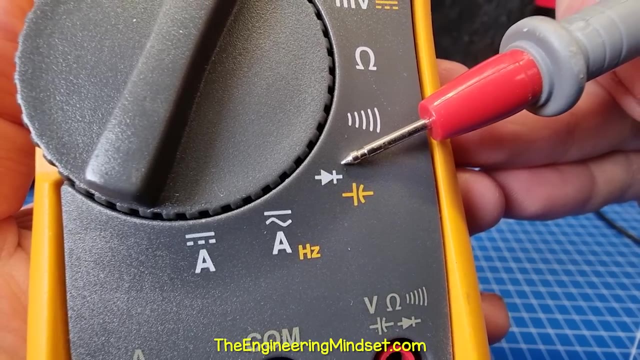 This particular meter defaults to AC voltage and indicates we need to press the yellow button to take a frequency reading. Diodes look something like this: They only allow current to flow in one direction. We use this symbol to represent them in engineering drawings. To test them, turn the dial to the diode setting. 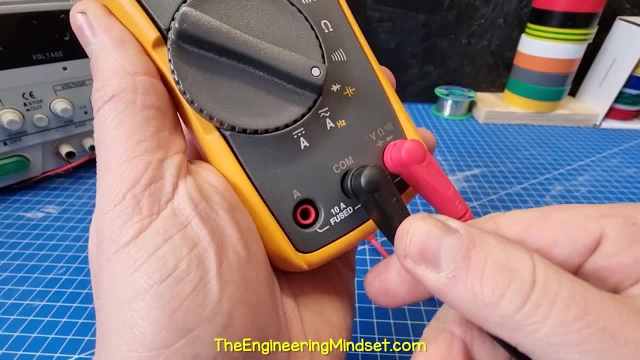 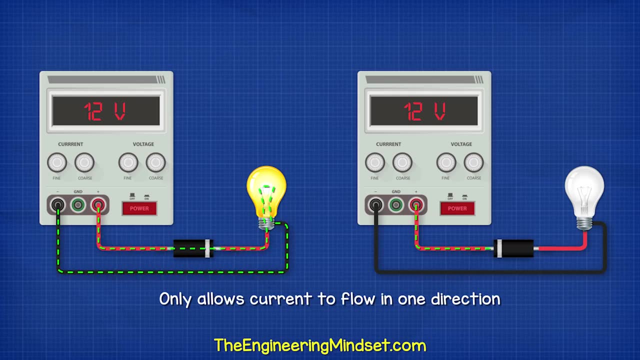 Connect the red lead to the diode terminal and the black lead to the COM terminal. If we connect the leads like this, we should read OL, because the diode has blocked the meter from taking a reading. When we reverse the line, we see that the LED is off. 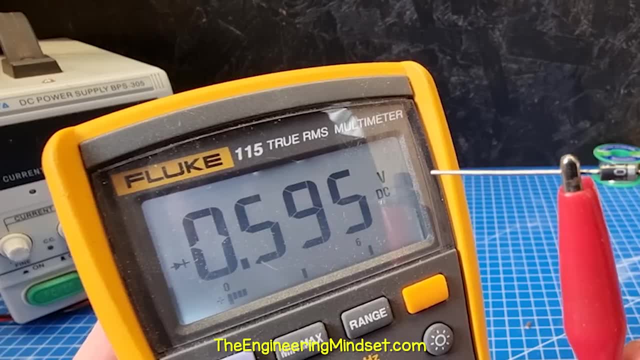 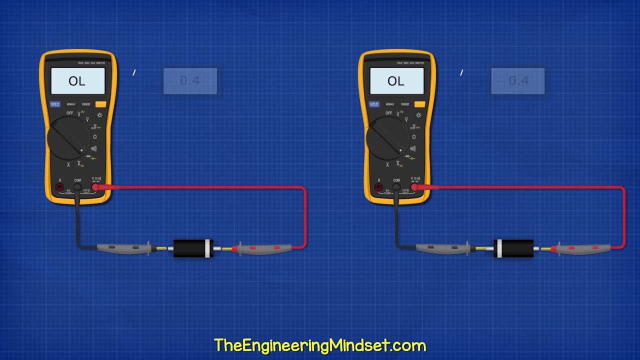 When we reverse the leads, a value should appear typically between 0.5 and 0.8.. If OL displays on both orientations or a reading of around 0.4 appears in both directions, then the diode is faulty and needs replacing. 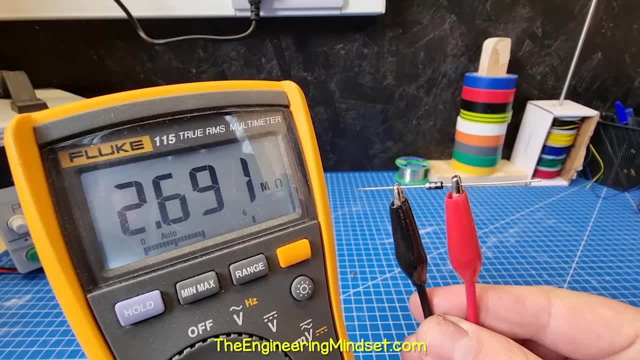 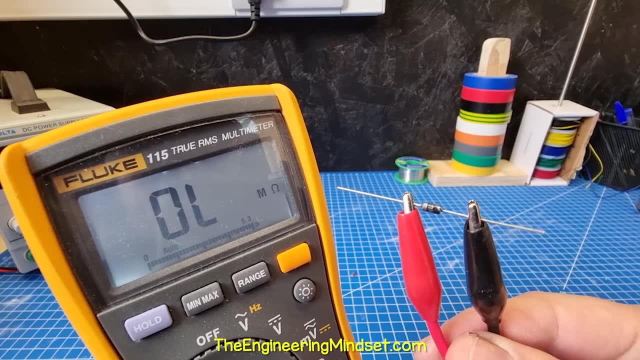 We can also check diodes with the resistance function. We should see a value of between one kilohm to 10 megaohms, and reversing the connections, we should just see OL. LEDs are also diodes. They just emit light. 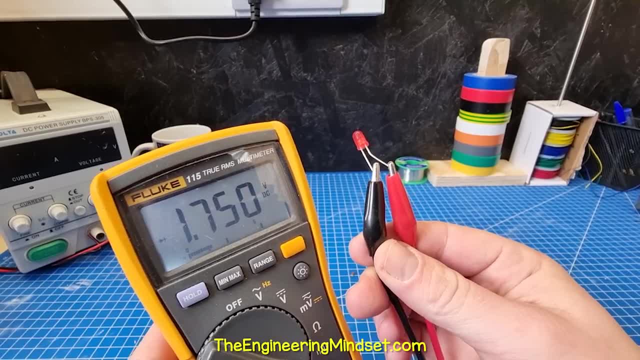 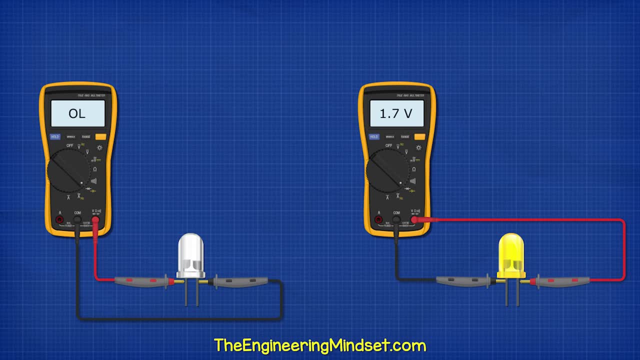 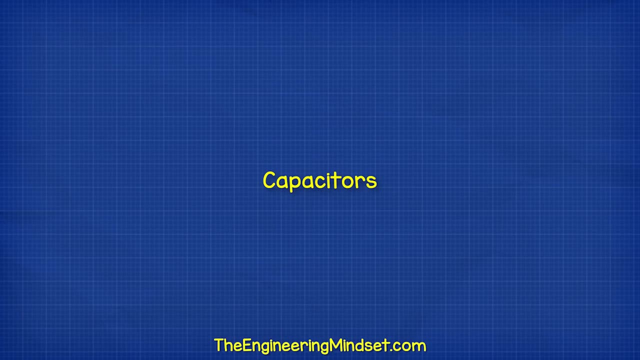 We can use the diode function to test these also. The LED should produce a dim light. LEDs only light in one direction and block the current in the reverse direction. Pi-voltage LEDs will not show a value. Capacitors store and discharge electrons within the circuit. 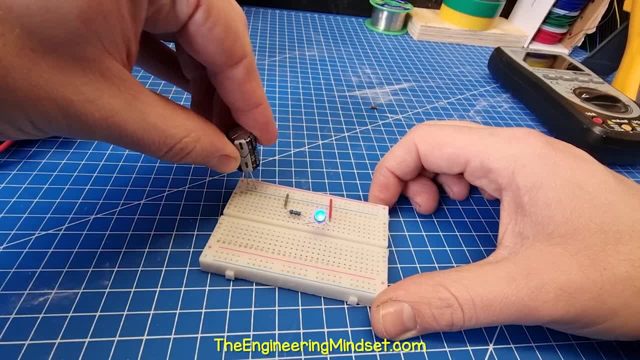 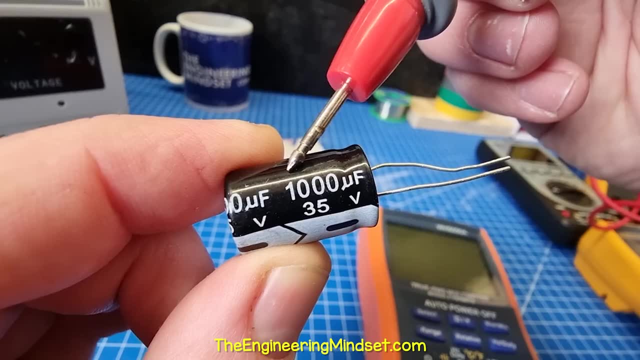 Capacitors store and discharge electrons within the circuit. They are represented with the L-shape. They are represented with the L-shape. They are represented with the L-shape On the side of electrolytic capacitors. it should state the rated capacity. 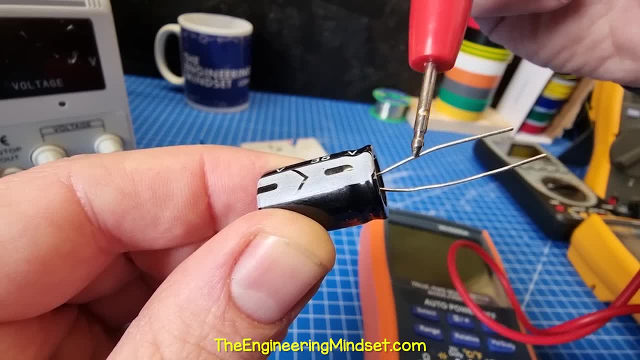 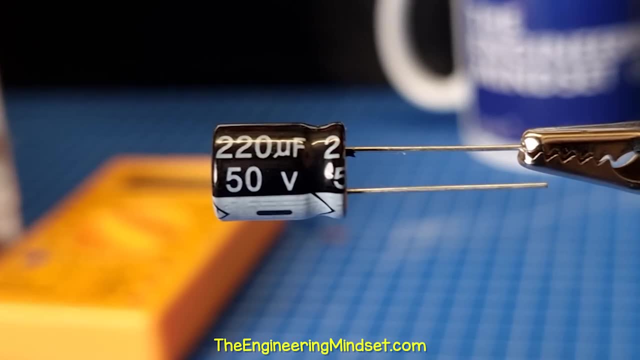 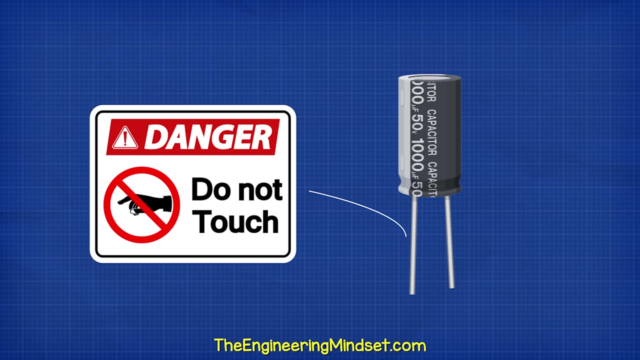 the maximum voltage and also the negative terminal. Some types do not display this. We would need to therefore find the manufacturer's data sheet. Capacitors can store high voltages for a very long time after they've been disconnected. Do not touch the leads, as it will discharge through you. 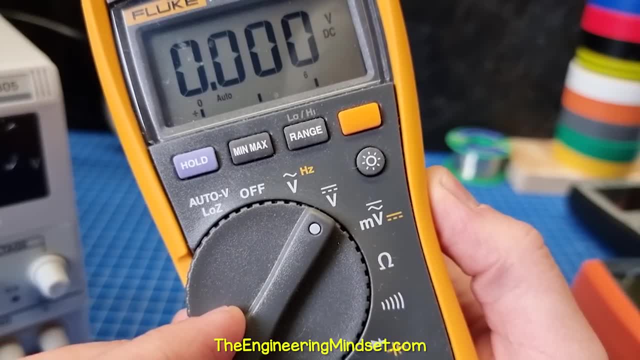 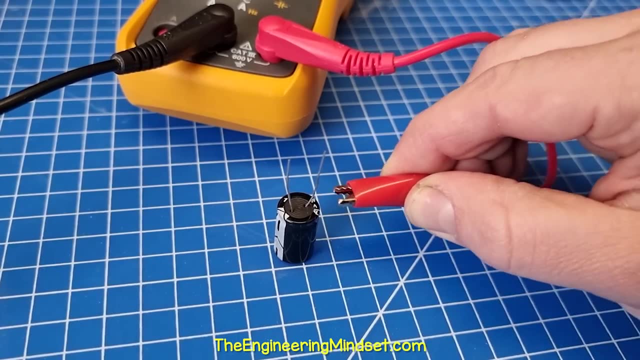 We can test the voltage of the capacitor by selecting the DC voltage. We can test the voltage of the capacitor by selecting the DC voltage. A very important factor is the voltage setting. Place the black wire into the COM terminal and the red wire into the V terminal. 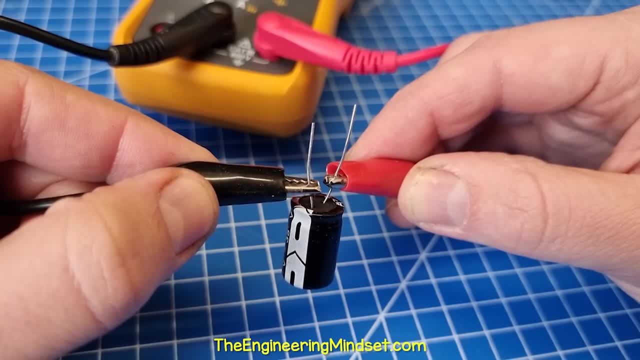 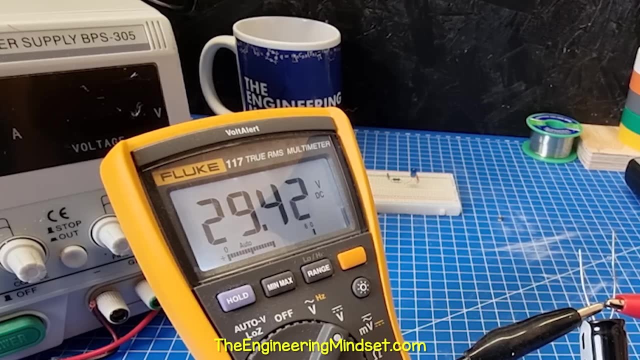 Then carefully connect the probes to the capacitor, with the black probe touching the negative terminal of a polarized capacitor, of a polarized capacitor. Not all capacitors are polarized. The meter will now display the stored voltage If we see a reading of several volts or more. 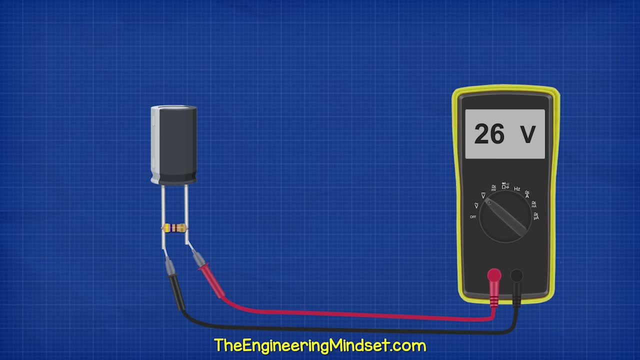 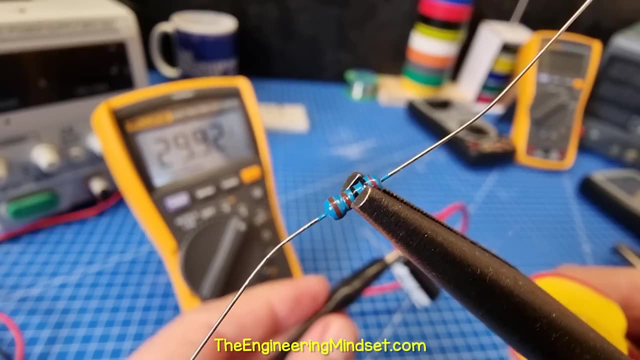 like this one, then we should place an appropriately sized resistor across the terminals. This is a small capacitor, So I will just use a two kilo ohm- 0.25 watt resistor, And then we can see the stored energy is safely discharged. 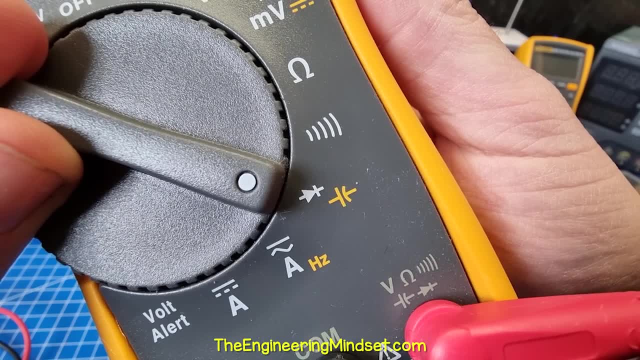 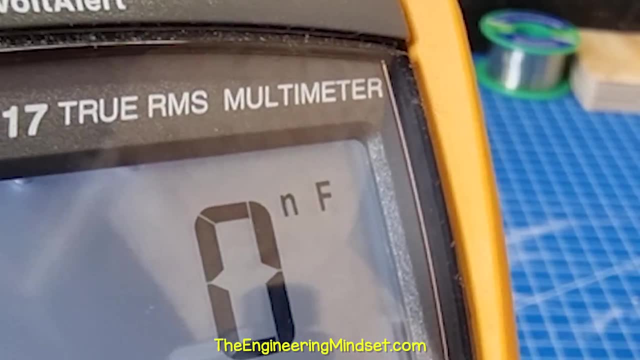 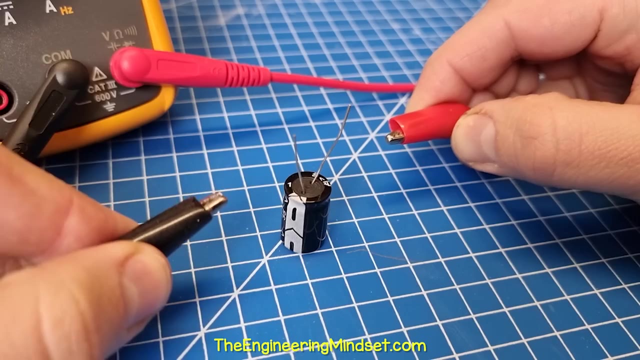 Now select the capacitor setting. This particular model defaults to diodes and indicates that we need to press the yellow button to switch to the capacitor setting. The black lead remains in the COM terminal and the red lead in the capacitor symbol terminal. Connect the black probe to the negative side. 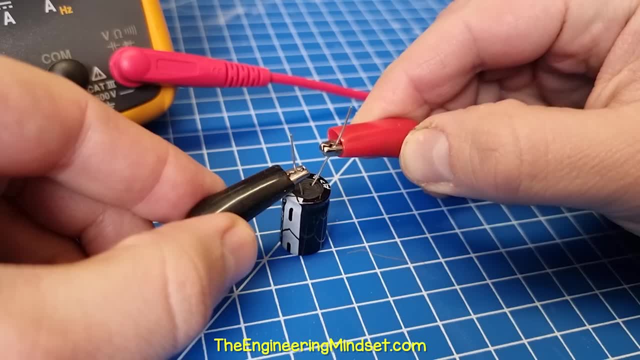 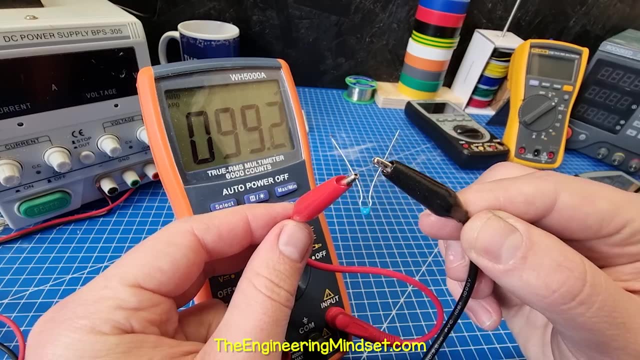 if polarized and connect the red probe to the positive side. It will then display the result. With non-polarized types, we can use the probes on either side. The result will probably not match the rated value. You can see here that this one is slightly higher. 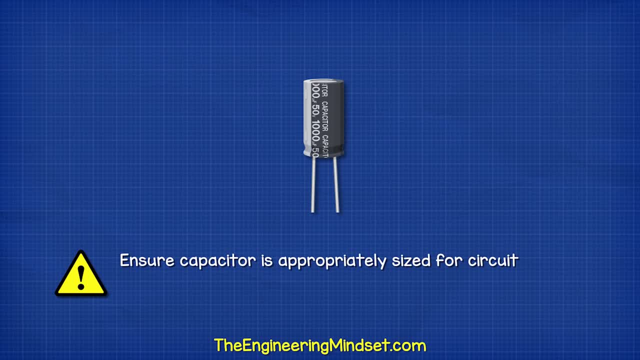 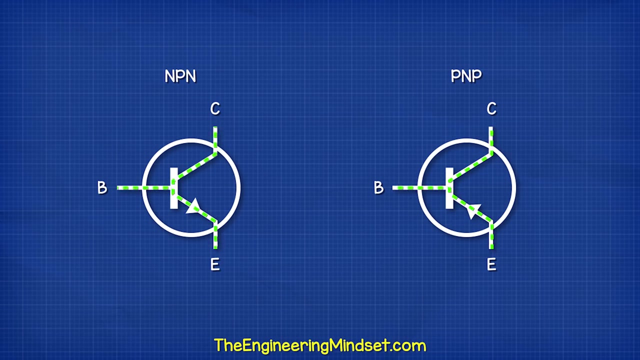 and this one is slightly lower. So we need to consider if they are appropriately sized for our circuit and we can exchange them if needed. Transistors load. They look like this And they are basically a type of electronic switch. They are represented by these symbols. 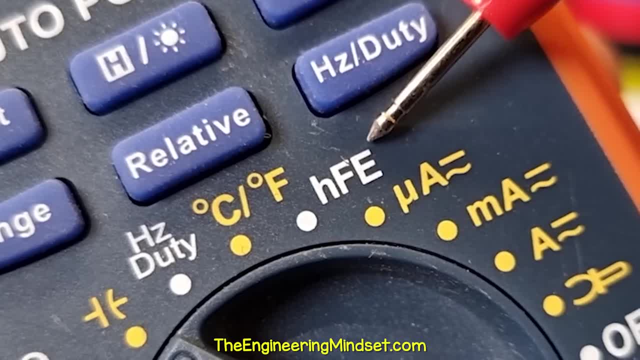 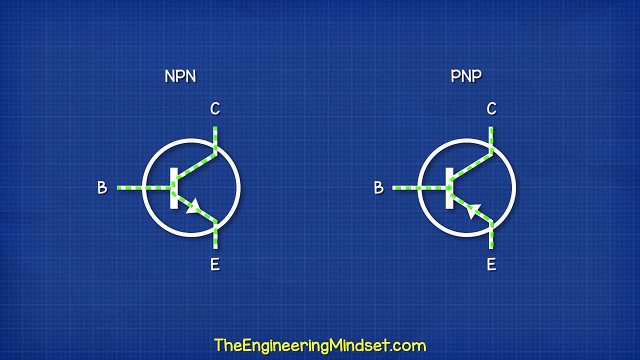 Although we use the HFE setting on a multimeter To test them. we locate the identification number on the front and then we find the data sheet for that. It will tell us here if this is an NPN or a PNP type. 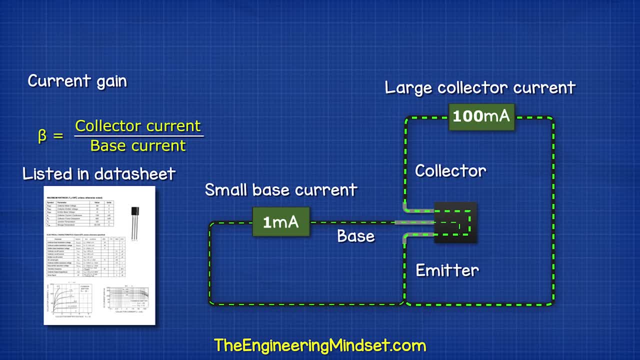 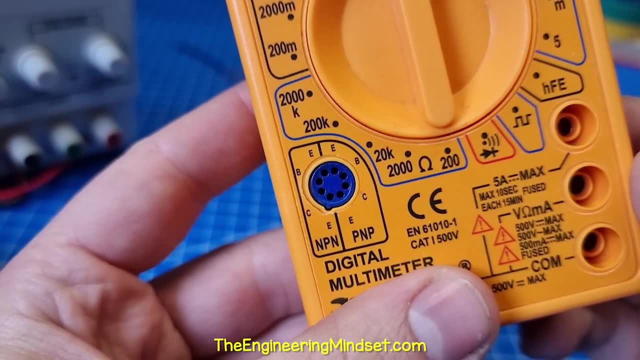 It will tell us which leg is the base emitter and collector and also the HFE value, which is the current gain. Next, We will need to locate the transistor test area on the meter. Sometimes we need an adapter like this one. We then select the HFE setting. 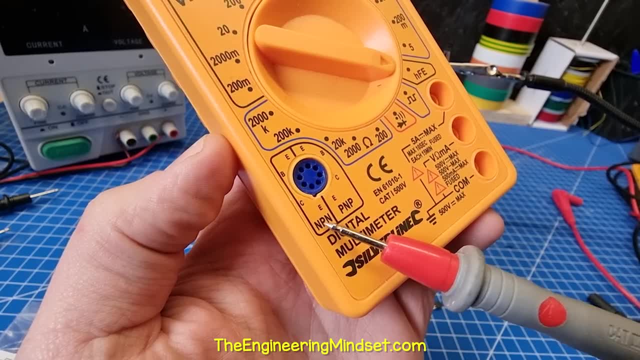 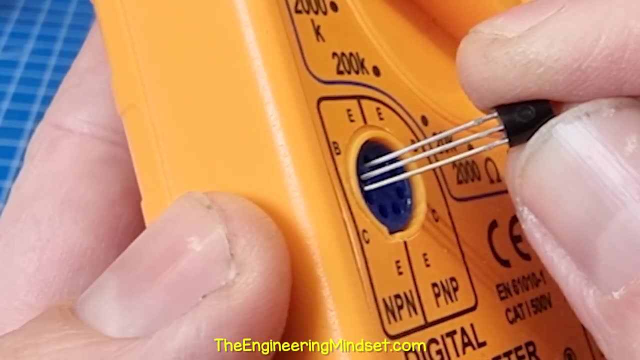 We then align the transistor with the type- For example, this is an NPN type, so I use the NPN side- And then we insert the legs into the correct terminals. The meter then displays the result. This one is within range, so it's good to use. 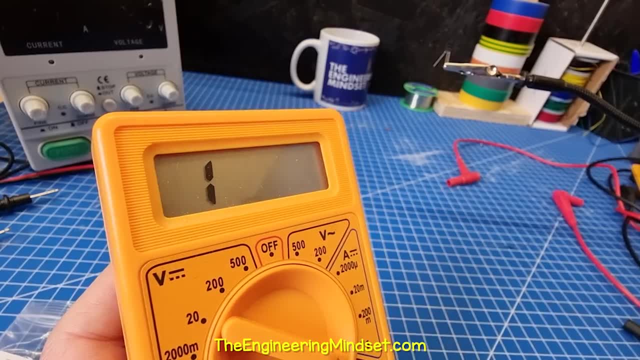 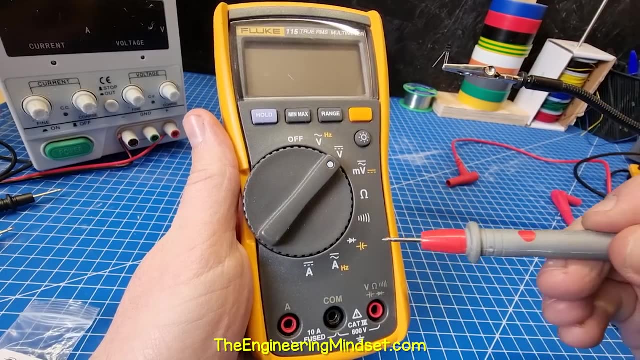 If the meter shows a value outside of this range or it displays just a 1,, then the transistor is faulty. If you do not have an inbuilt transistor tester, then we can use the diode setting. Insert the red lead into the terminal with the diode symbol. 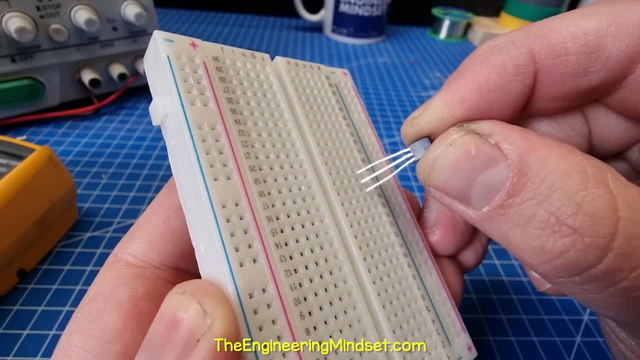 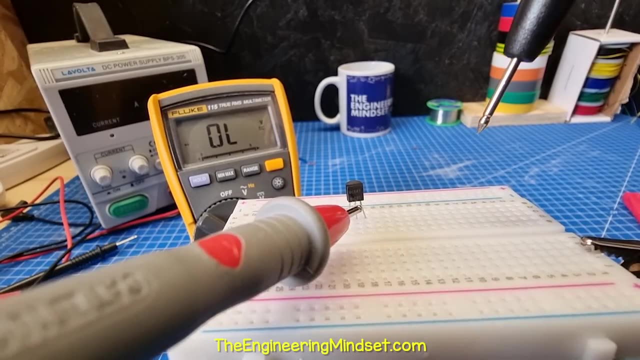 and the black lead into the COM terminal. Then insert your transistor into a test board. We already know that this one is an NPN type, so we place the red lead on the base pin And we will then see a reading of around 0.6 to 0.7.. 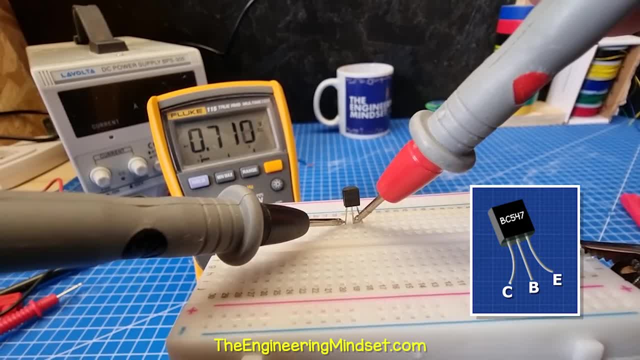 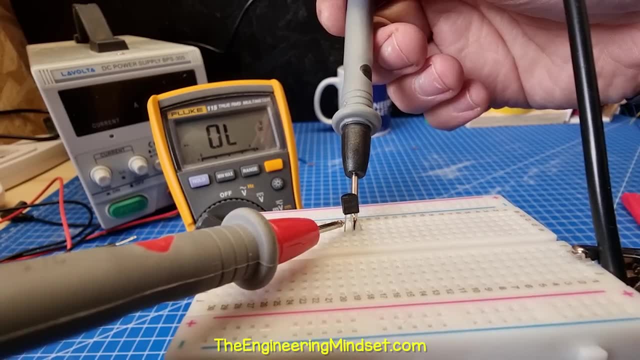 And we will then see a reading of around 0.6 to 0.7.. When we connect to either the emitter or the collector, It should not give a reading if we test across the emitter and collector, Or if we place the black probe on the base and then test the emitter or collector. 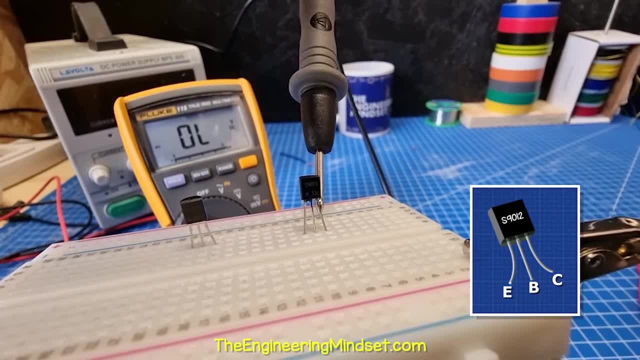 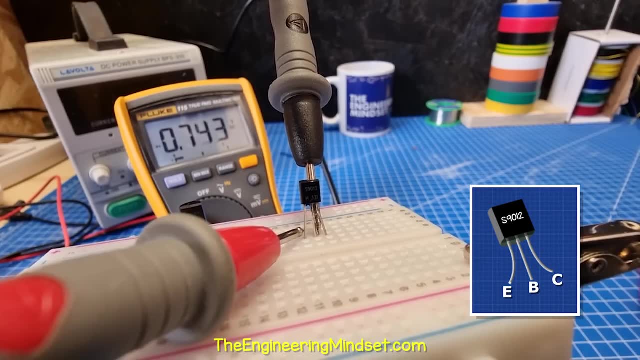 This one is a PNP type, so we need to place the black probe on the base pin. When we place the red probe on the emitter or collector, we should see a reading of between 0.6 and 0.7.. We should not give a reading of around 0.7.. 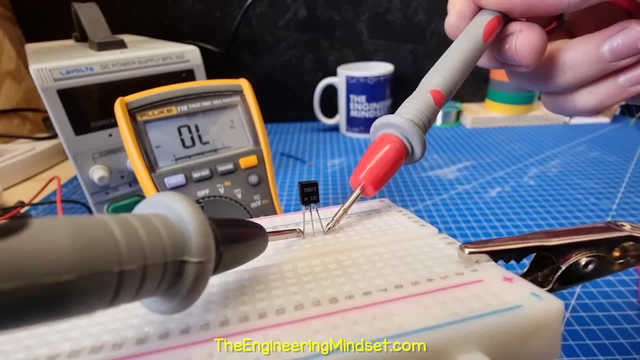 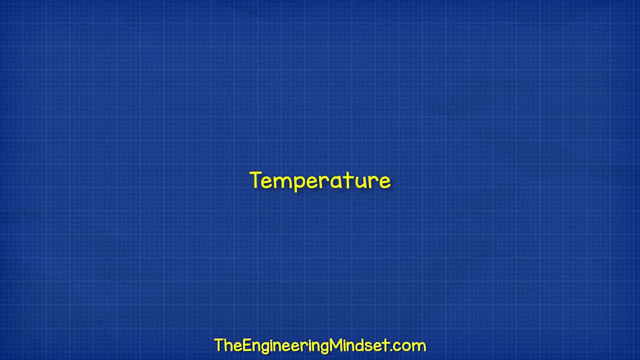 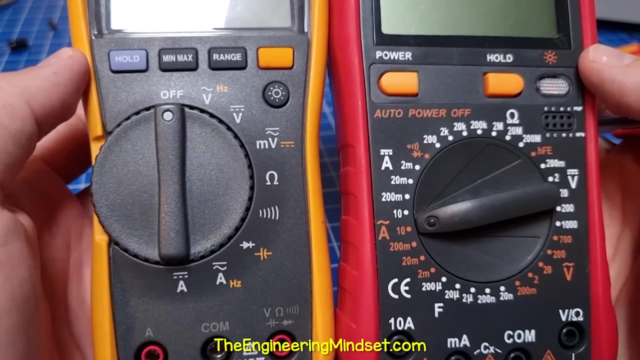 We should not see a reading if we test across the emitter and collector, Or if we place the red lead on the base pin and test the emitter or collector. This is the symbol for temperature reading. Although not all multimeters have this, It's very simple to use this feature. 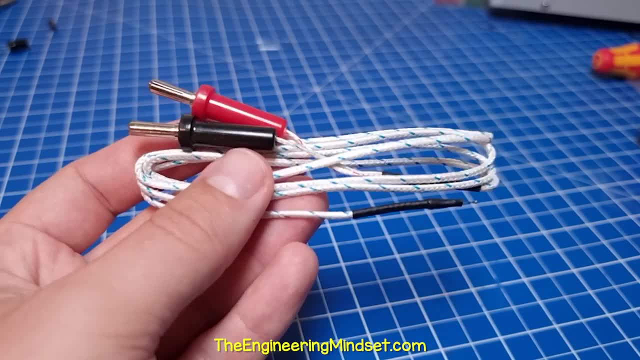 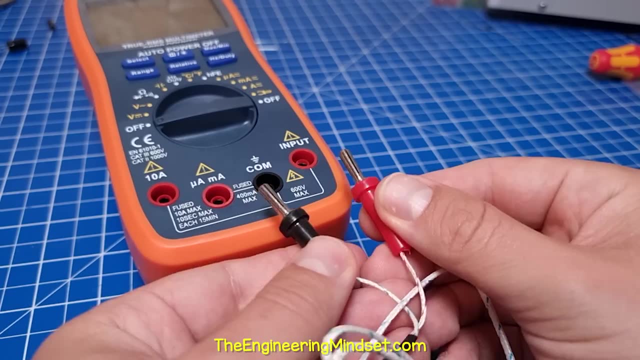 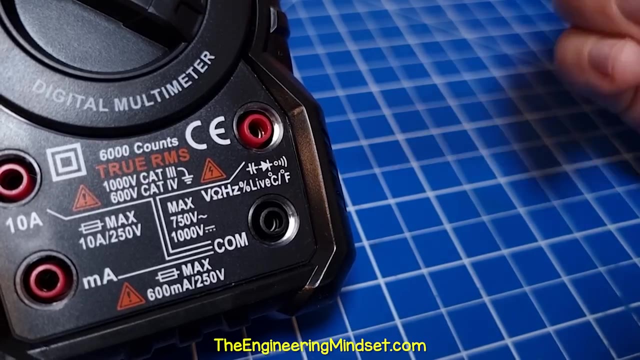 We just find our temperature probe, which typically looks like this, with the thermal couple at one end and the connectors at the opposite end. Ensure that the connectors are connected to each other. Ensure that the connectors are inserted with the correct polarity. Place the black lead into the COM terminal and the red lead into the terminal marked with the temperature symbol. 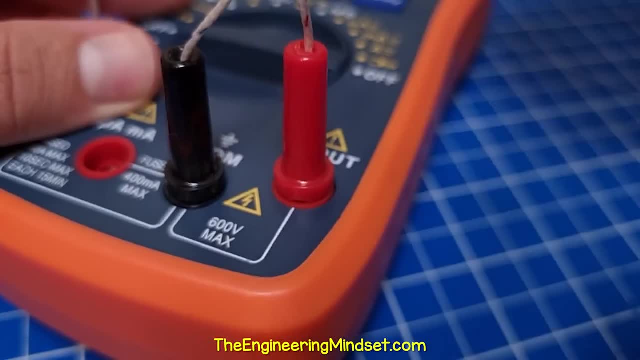 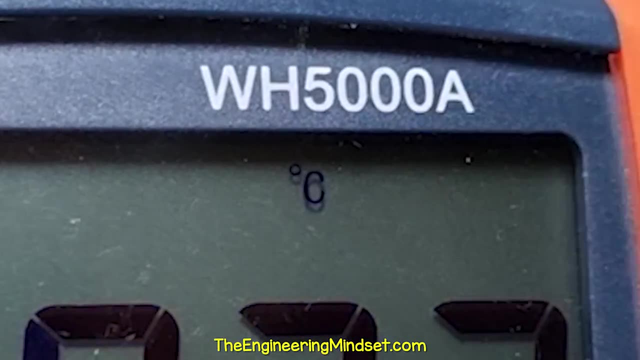 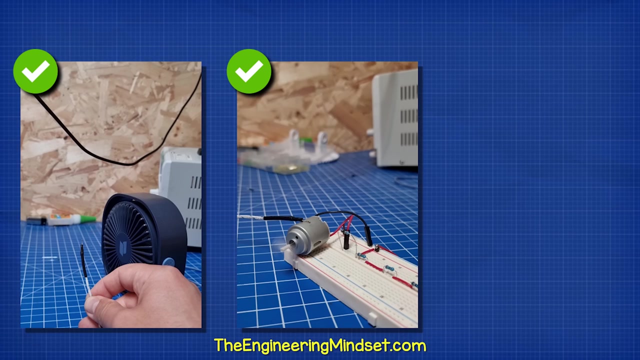 Although this one just says input, but we can still use this terminal- Then select the temperature setting on the meter. It will then display the result. This one defaults to Celsius, but we can change the Fahrenheit just by pressing the button. These probes are used for air temperature or surface temperature only. 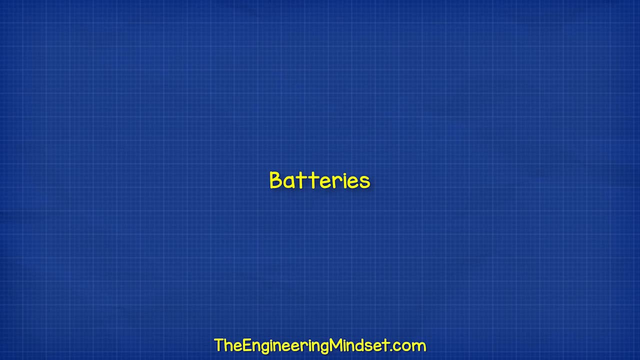 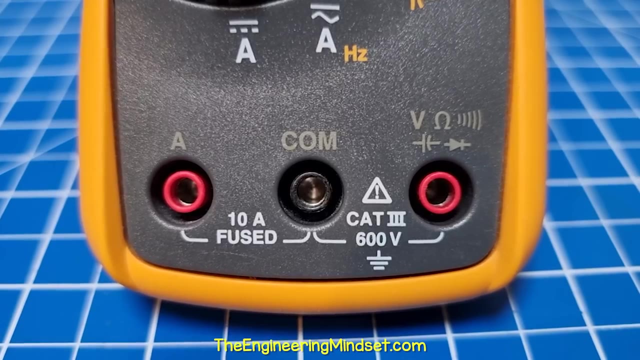 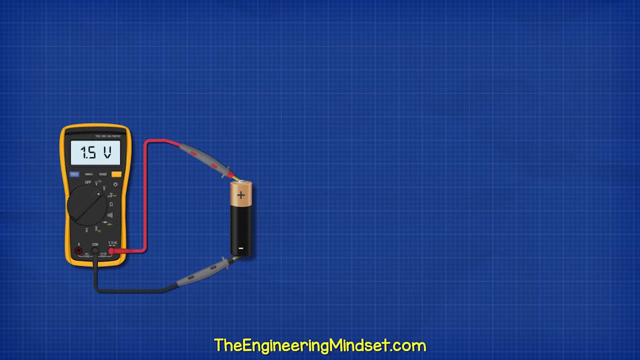 Do not use them in water. We need to test a battery in two ways. First, place the red lead into the V terminal and the black lead into the COM terminal, Then select the DC voltage setting. We connect the red probe to the positive terminal and the black probe to the negative.